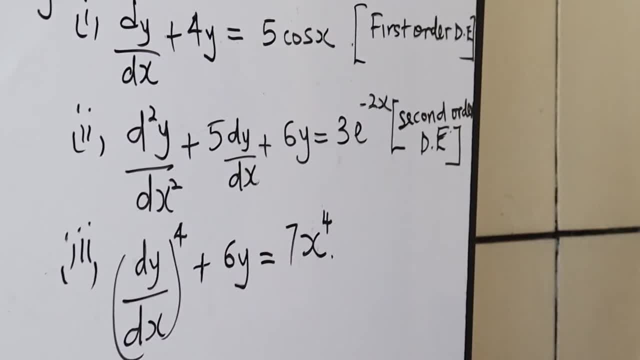 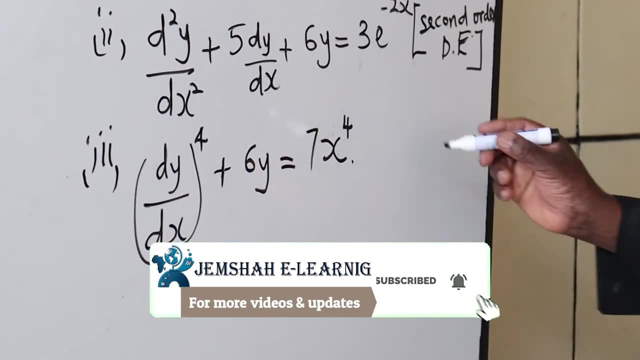 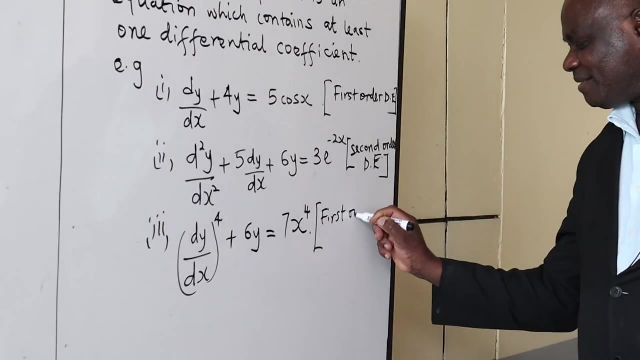 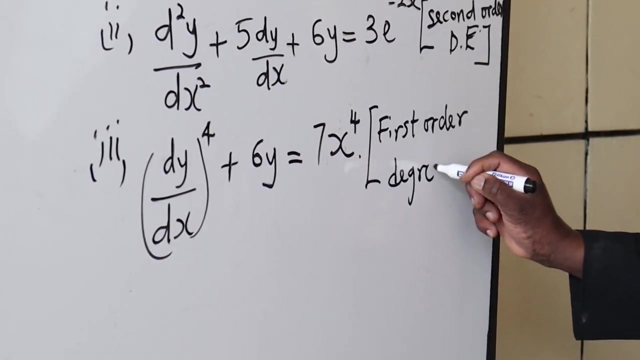 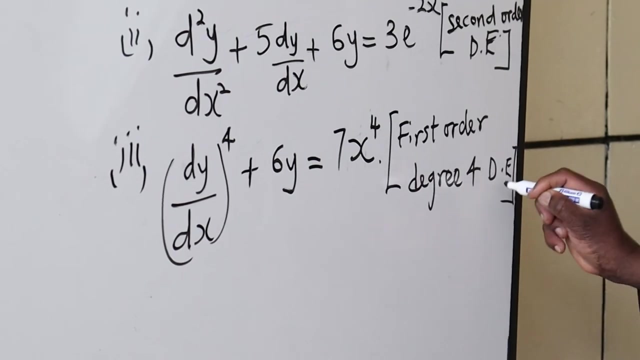 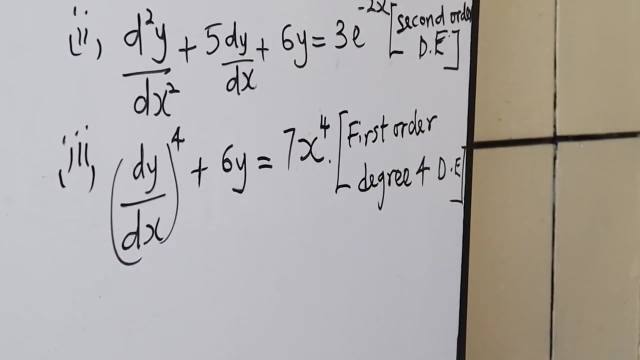 Now the third one. the highest derivative is first derivative, but it is put to power 4.. So this one we'll call it first order differential equation. First order degree 4 differential equation. First order degree 4 differential equation, because it is put to power 4.. 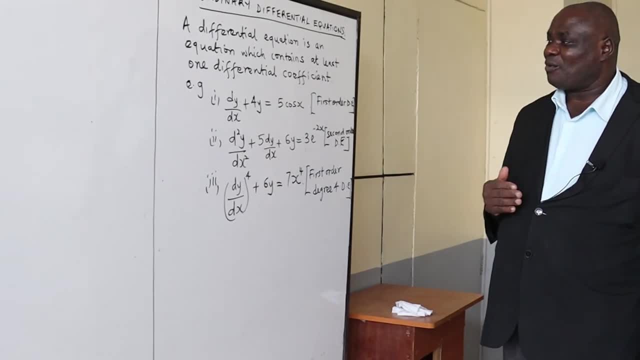 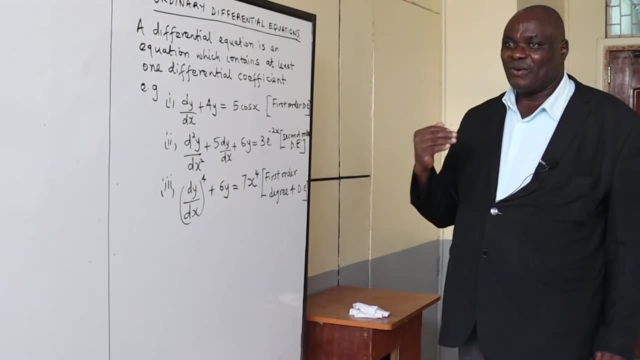 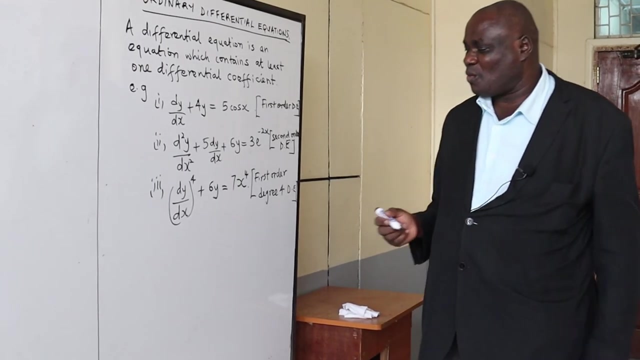 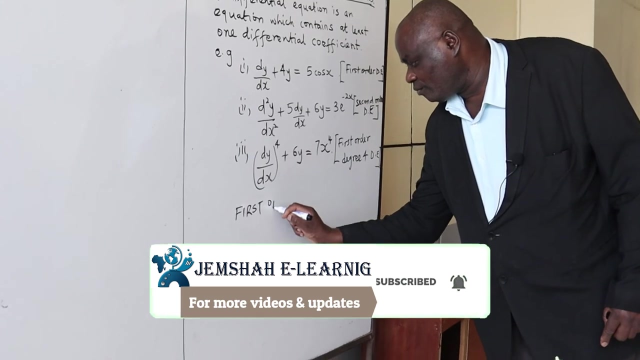 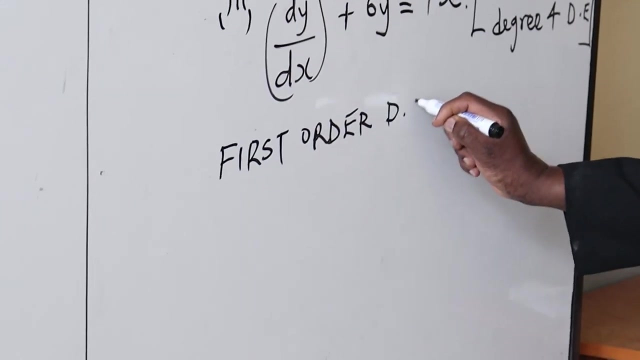 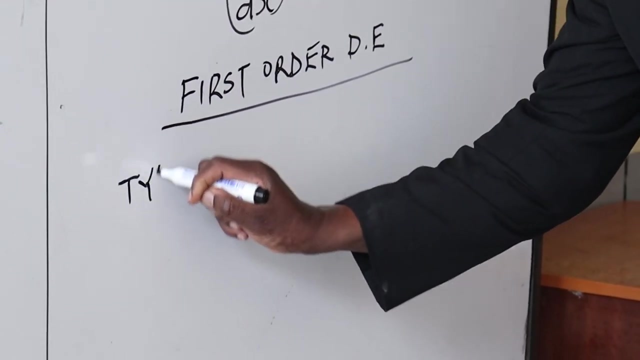 After this, then, we need now to tackle first order differential equation. First order, ordinary differential equation. Second order: ordinary differential equations. Now we are going to start from first order differential equation. First order, First order, the differential equation, And we are starting with the type 1.. 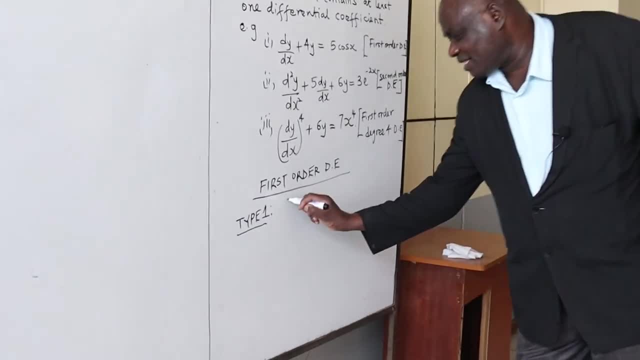 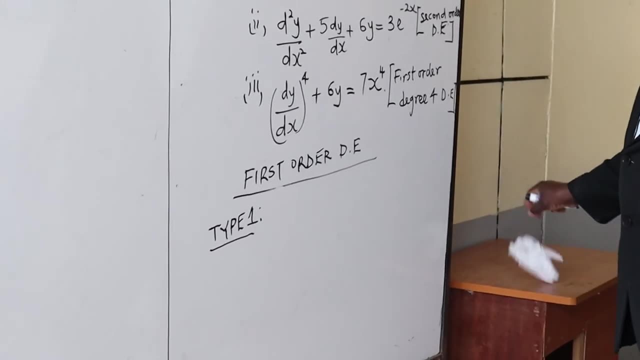 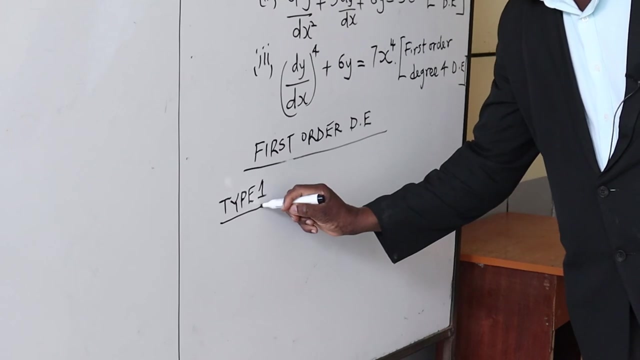 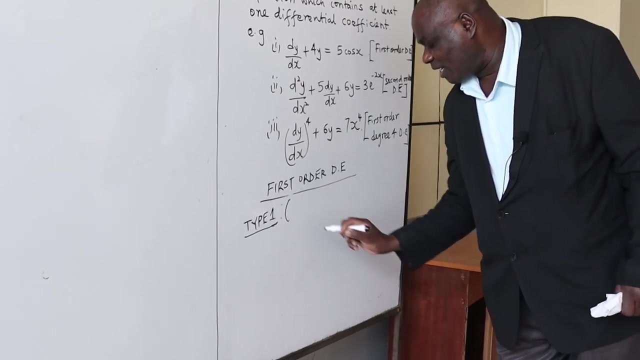 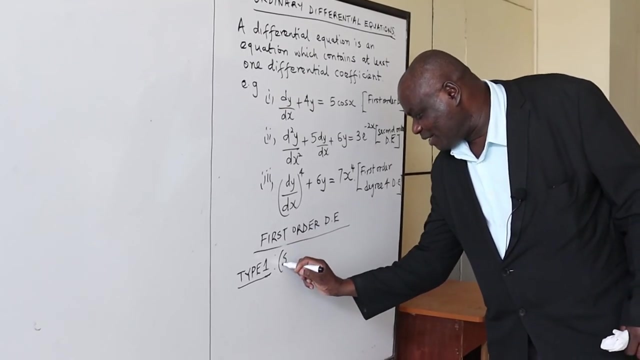 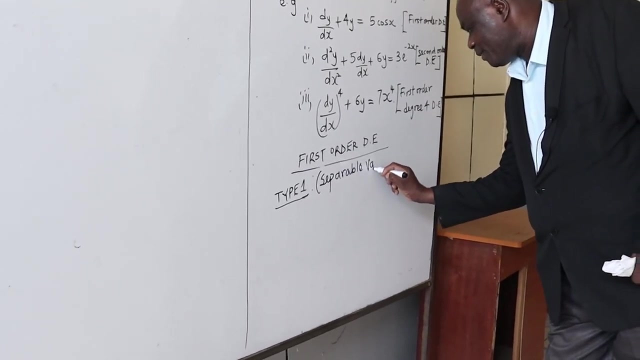 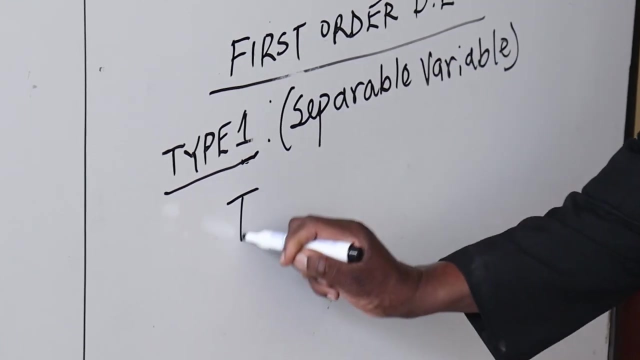 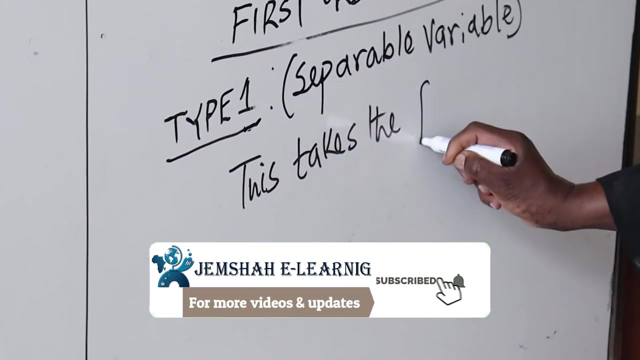 Type 1. This takes the form. We are going to call this one using the method it is being used to solve. So, first order, differential equation. So we will call it separable variable And we say: this takes the form, This takes the form. 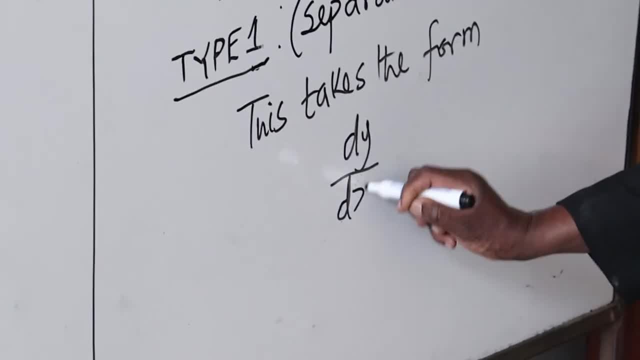 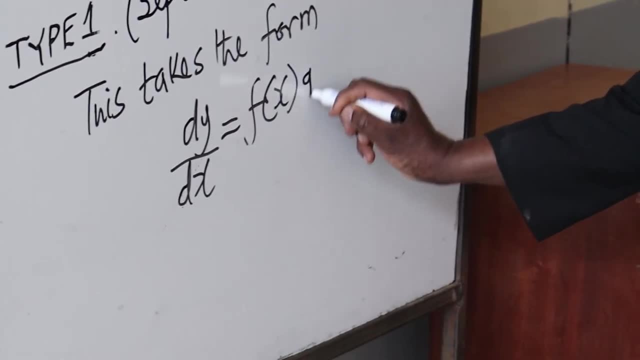 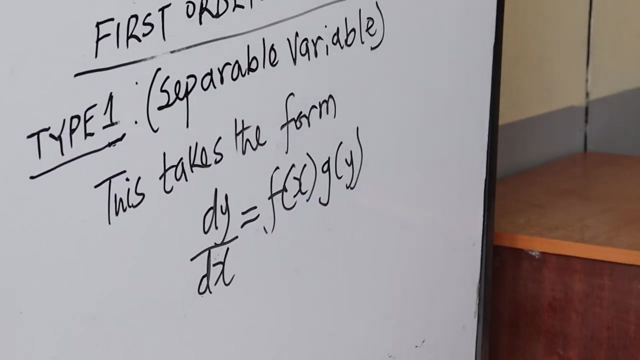 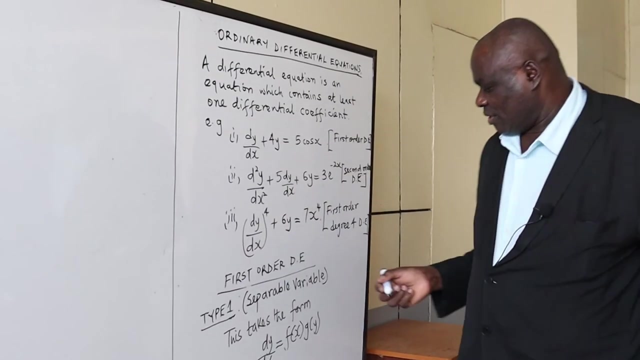 dy dx. This equals to function of x multiplying another function of y. So dy dx will be equal to f of x, g of y, f of x, g of y. So in solving this, we will solve by separating the variables. 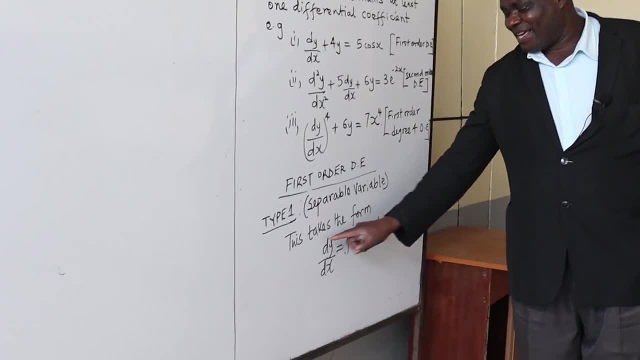 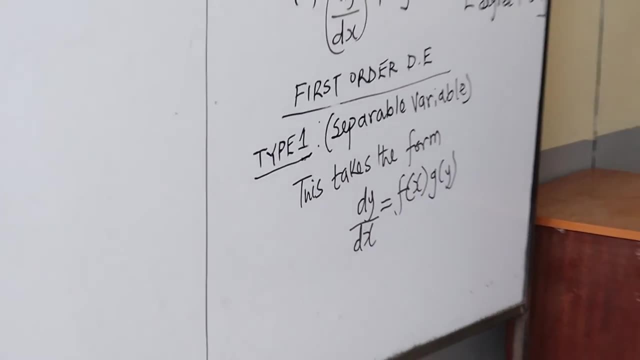 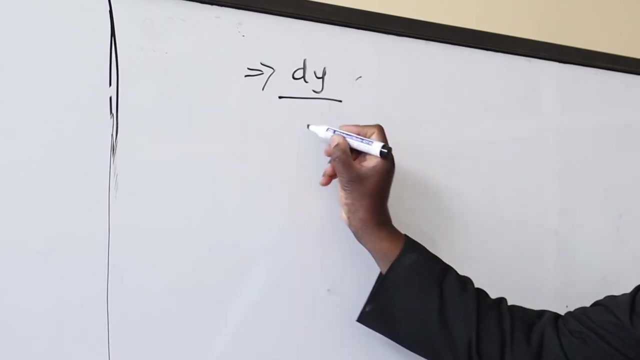 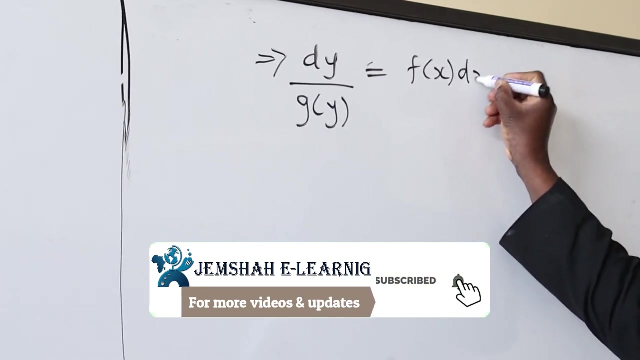 A function of y should be taken where there is a dy And now dx to join where we have function of x. Now this implies dy all over g of y will be equal to f of x, dx Will be equal to f of x dx. 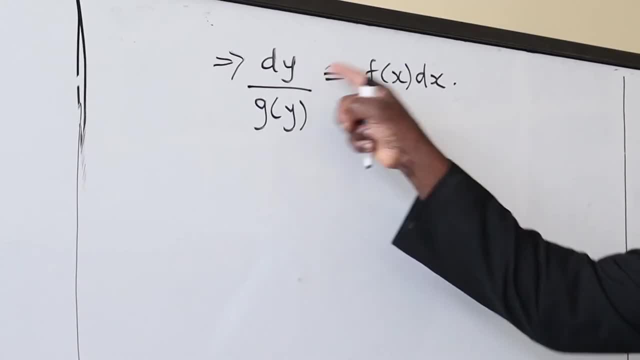 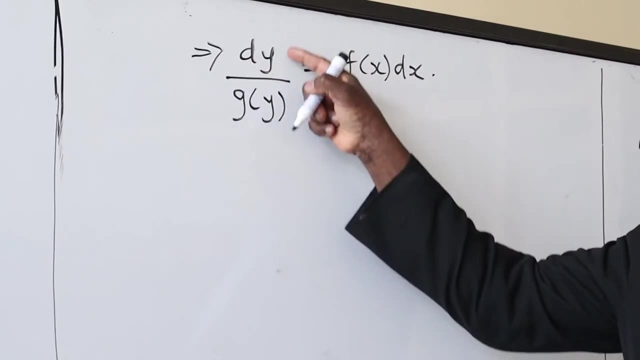 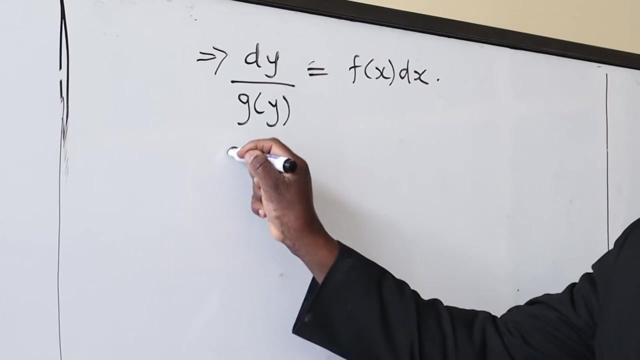 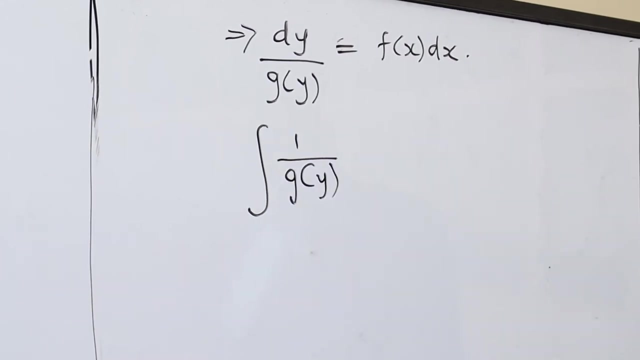 Now From this. we need now to solve for y And for us to remove the differential coefficient dy or dx. After separating the variables, we can integrate both sides With respect to the variable concerned, So that we can be able to get y. 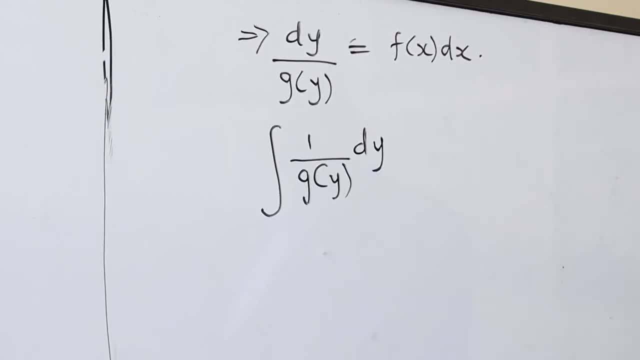 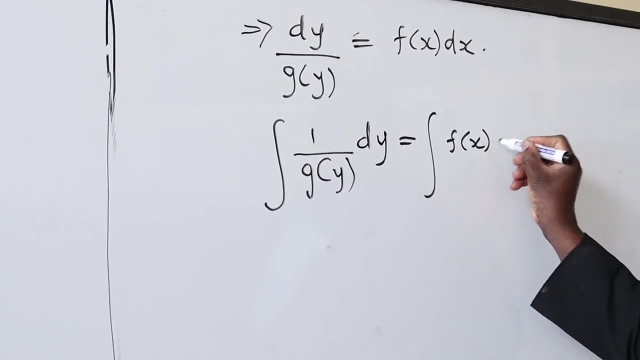 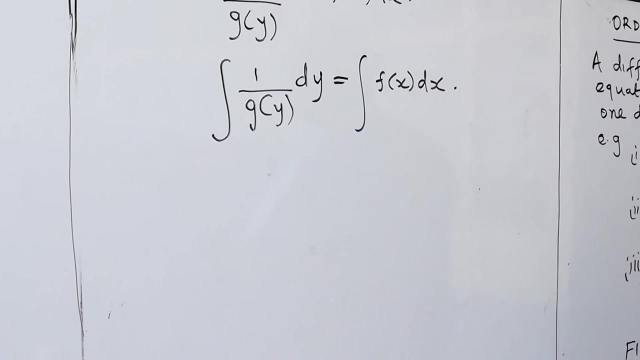 Get y as a solution. So the integral of 1 all over g of y dy Will be equal to the integral of f of x dx, f of x dx, And by doing so we can now make y the subject, Or we will have gotten the solution of that particular differential equation. 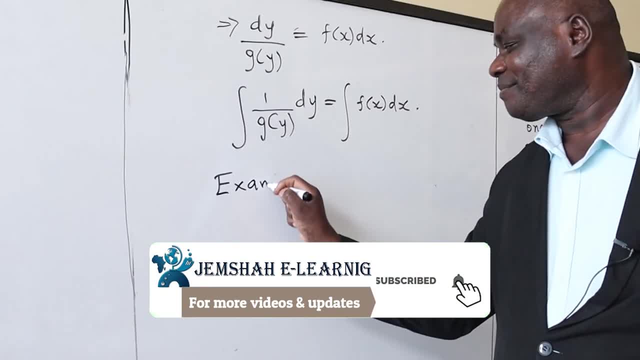 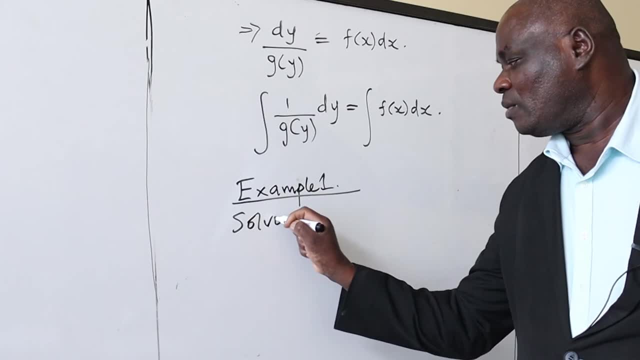 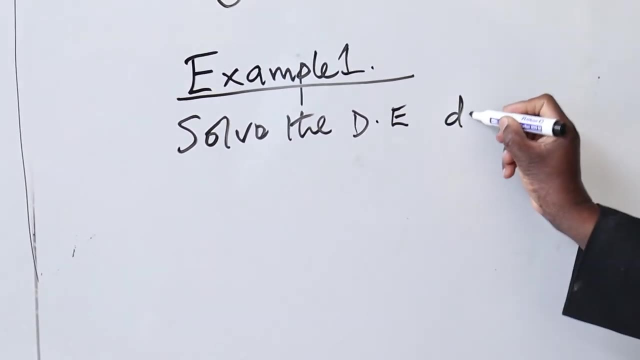 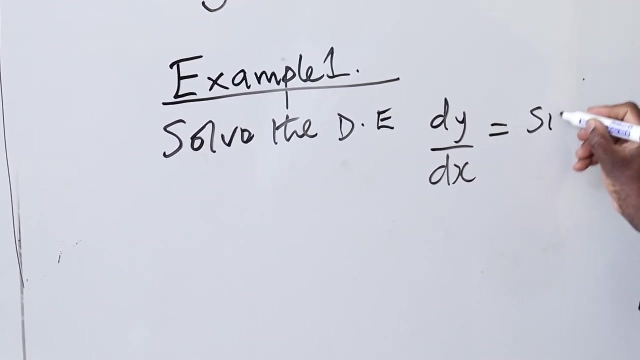 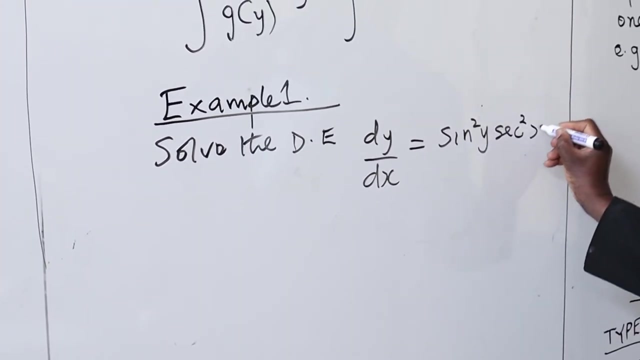 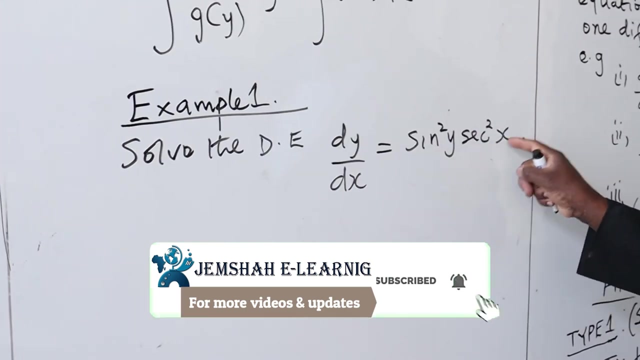 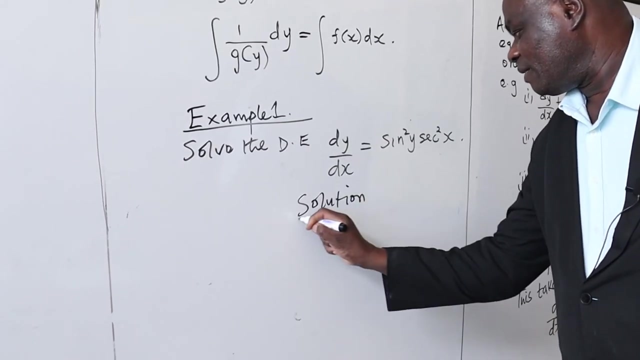 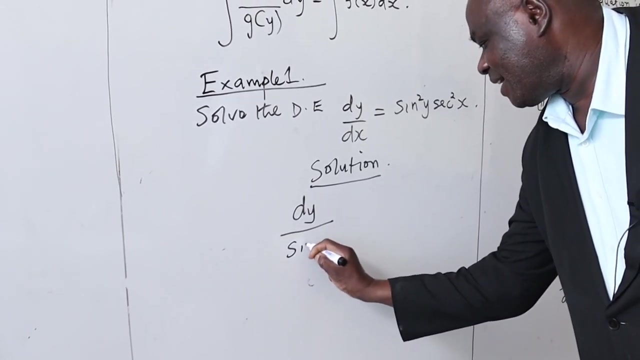 So, example one: Solve the dy, Solve the dy. dy dx is equal to sin squared x, x squared x. So in our solution, In our solution, this will be dy dy all over sin squared x, sin squared y, dy all over sin squared y. 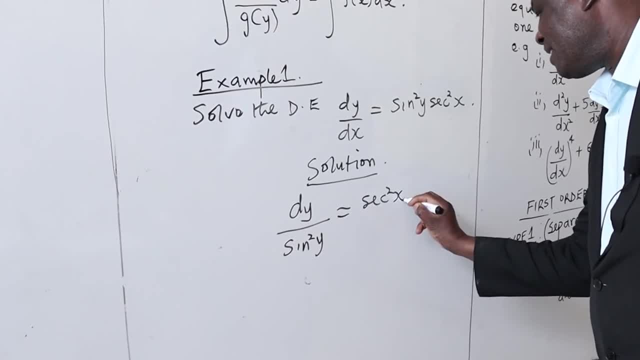 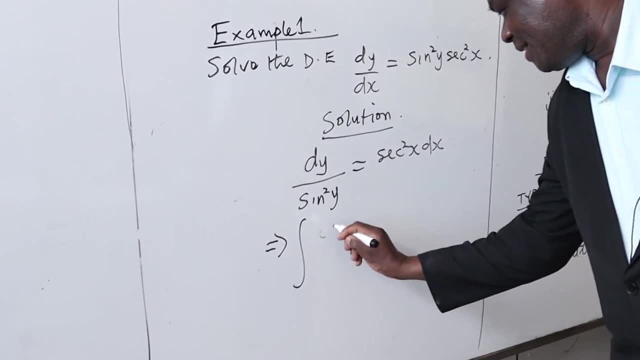 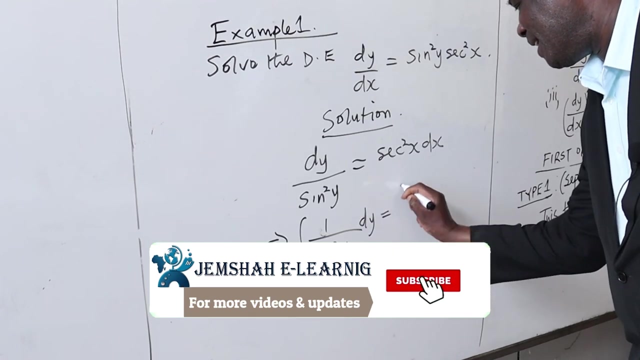 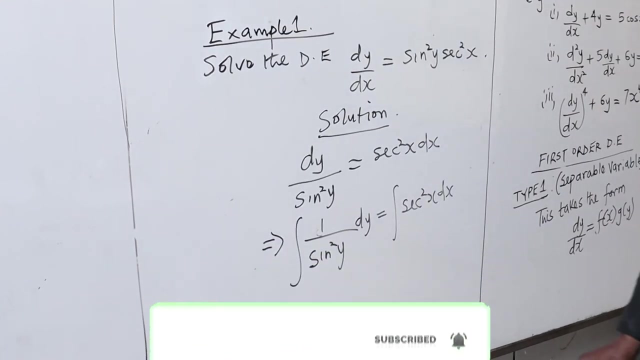 Will be equal to sec squared x- dx. This implies The integral Of 1 all over sin squared y. dy is equal to the integral Of sec squared x- dx. Now This implies also The integral 1 all over sin squared y. 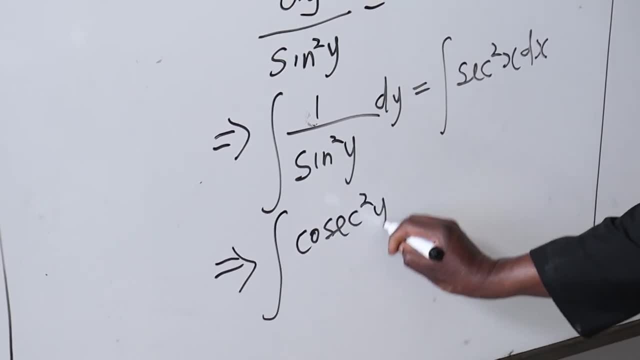 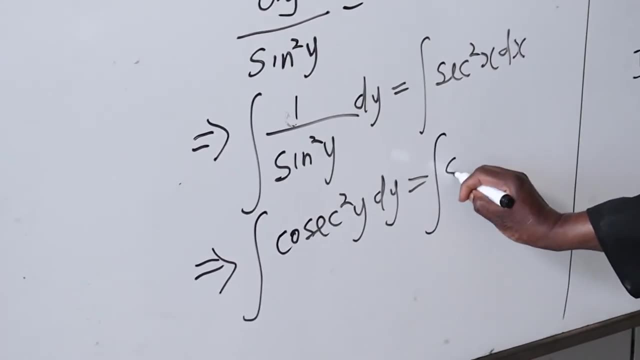 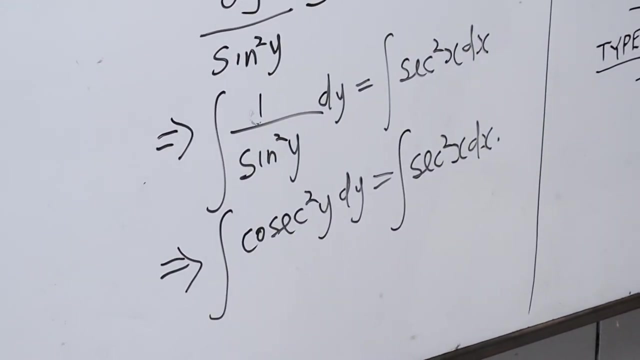 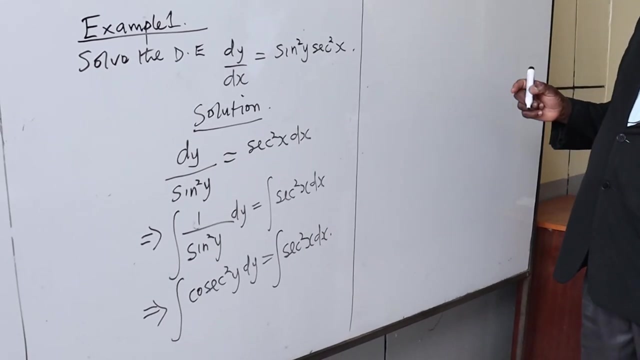 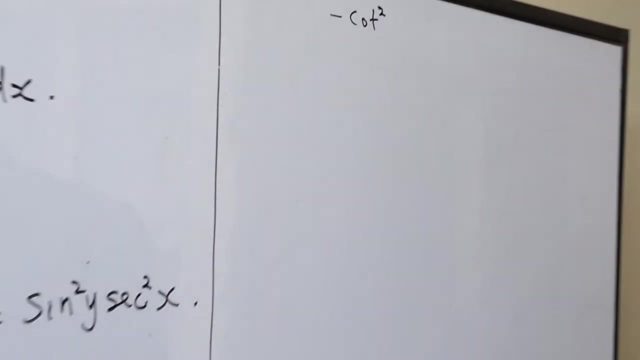 Is called sec squared y dy, Which will be equal to The integral of sec squared y. sec squared x. Now, in integrating this, The integral of sec squared y dy Will be minus squared dx. It will be minus. 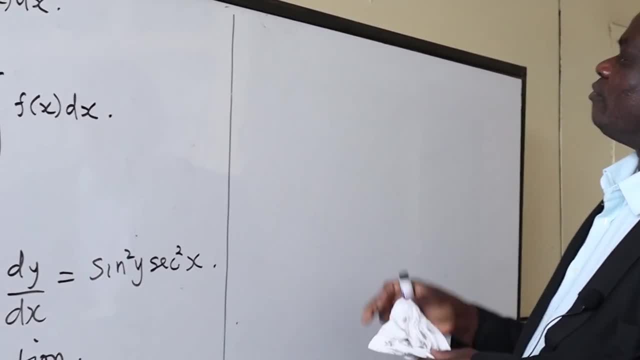 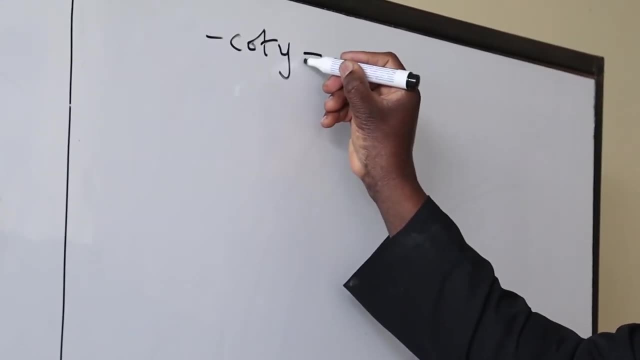 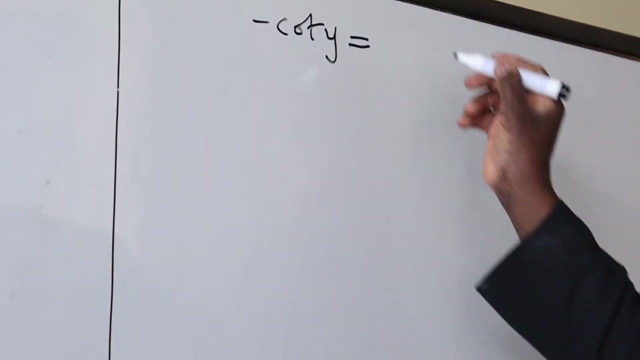 squared y, Which will be equal to, Which will be equal to, Which will be equal to. The integral of sec. squared x Is equal to tan x. Now, Since these were definite Integrals, The integral of sec squared x. 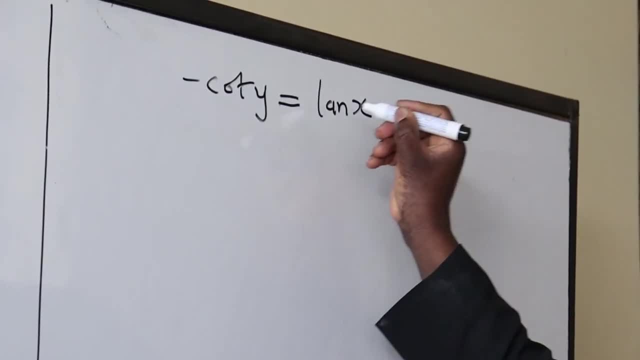 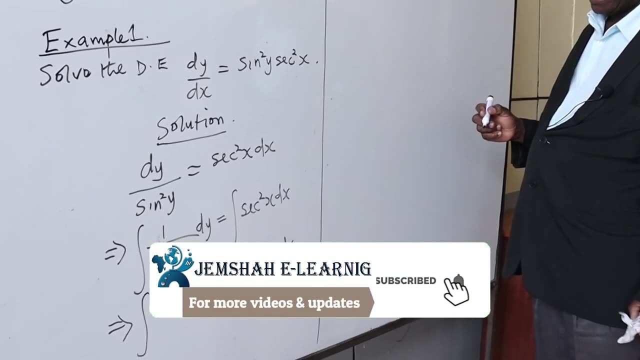 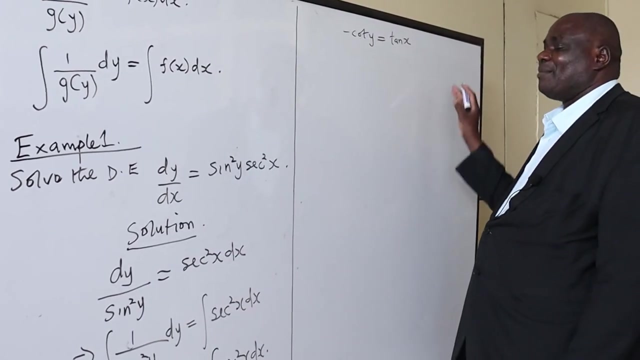 is equal to tan x. Now, Since these were definite Integrals, Each side attracts A constant of integration, And now We would like One constant Added to another constant, Or one constant Subtracted from another constant Will just be equal. 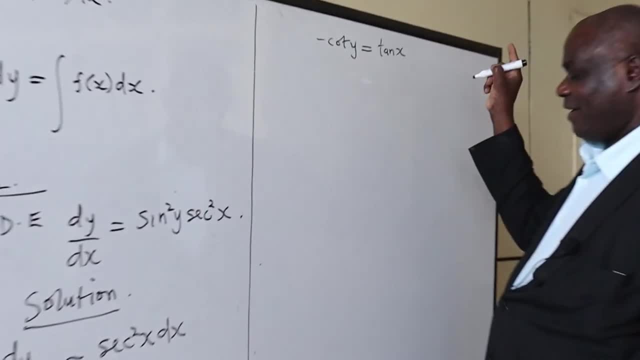 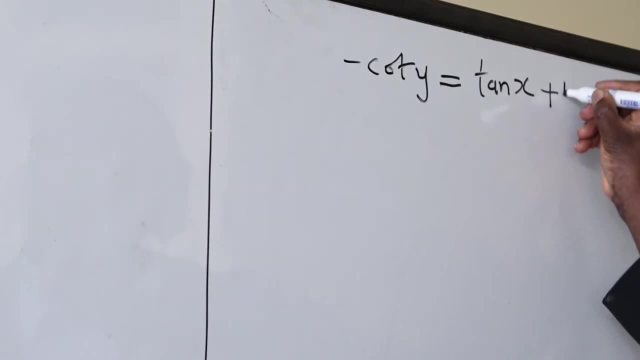 To a single constant, So we can include A constant of integration On our right hand side. So we say: Plus A constant k. So Minus squared y Is equal to sec, squared y, dx, dx. 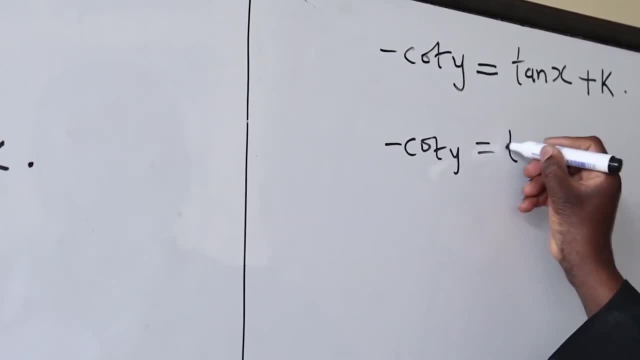 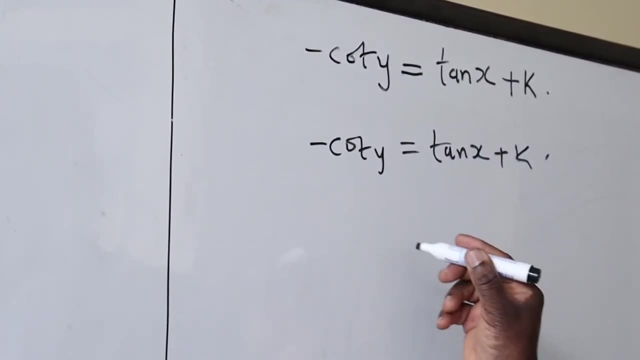 squared y Is equal to tan x Plus k, Which can also be written As: Which can also be written As: tan x Plus squared y Is equal To a constant k, And that is the solution. 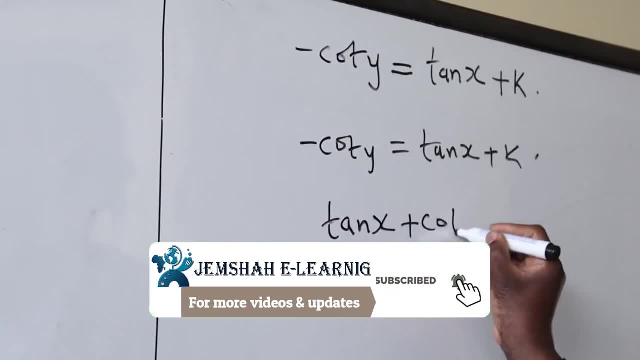 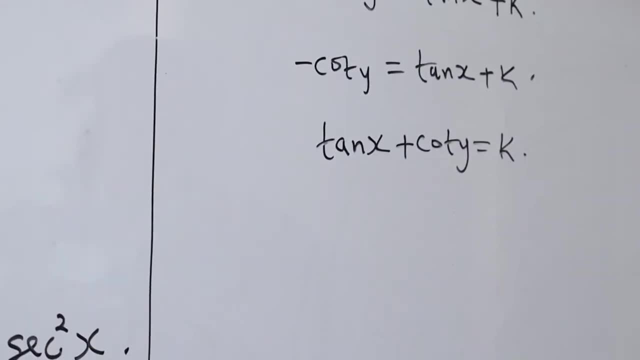 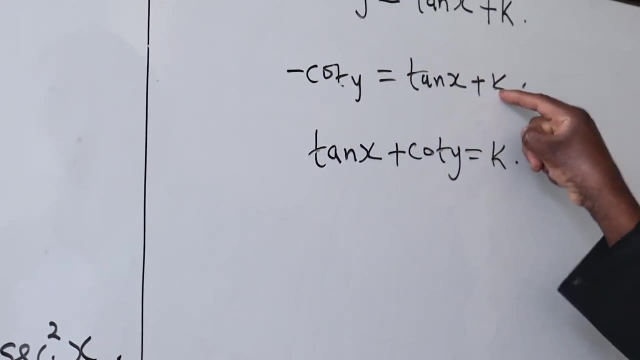 To that differential Equation Is equal To x, Because sec squared y Is equal to a constant k And that is the solution To that differential. Because If We Take This: 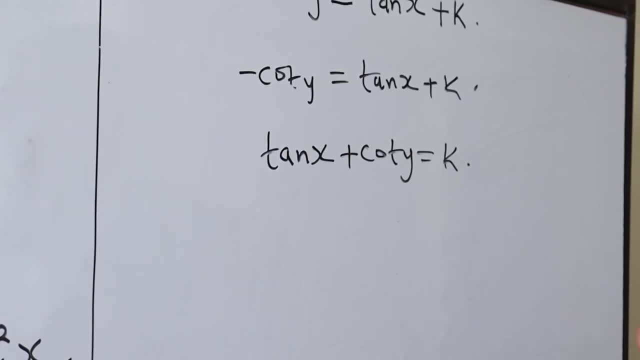 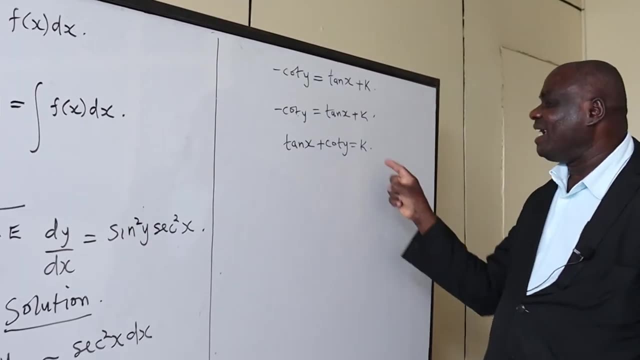 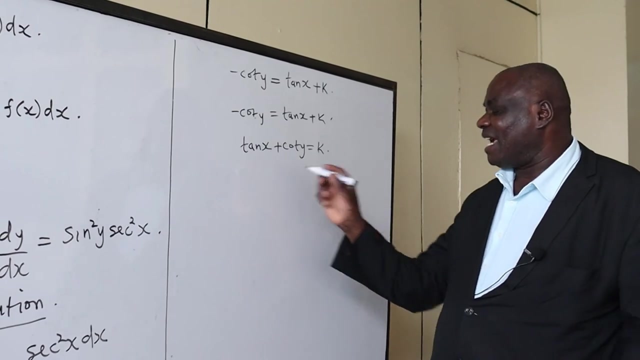 One Here And We Move k To This Other Side. k Will Be Minus k, But A Minus k Because We Still Don't Know. 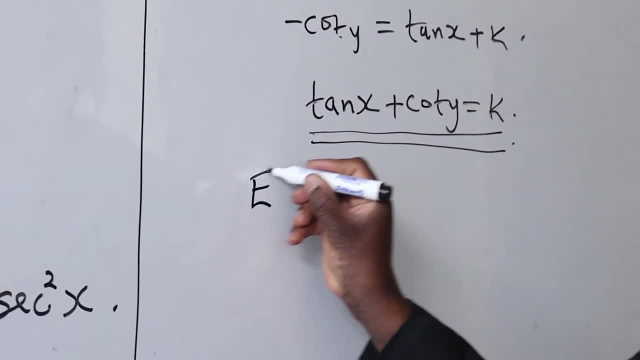 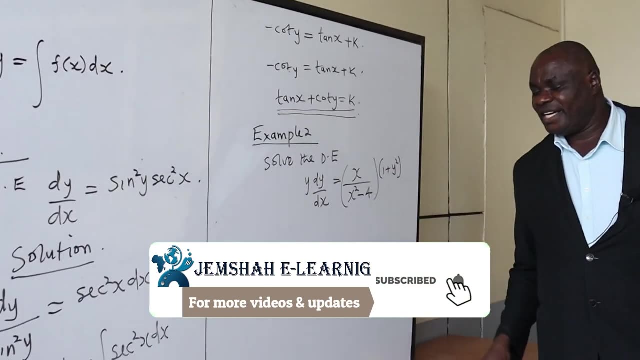 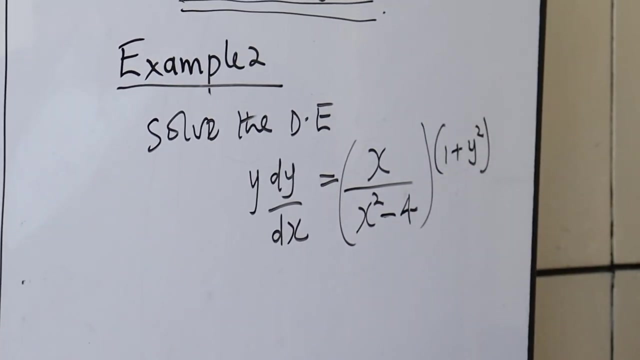 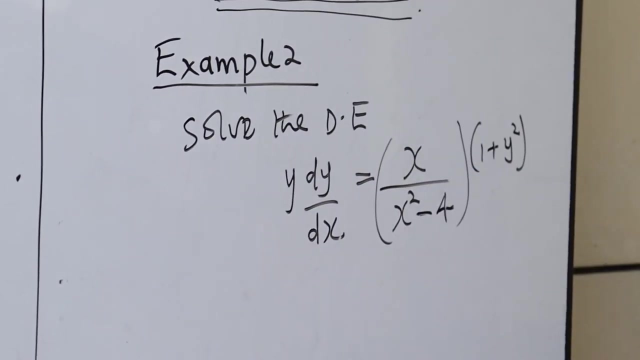 So We Move To Example Two. So Some Of The Y, D, Y, D, X Is Equal To X All Over X Square Minus Four. 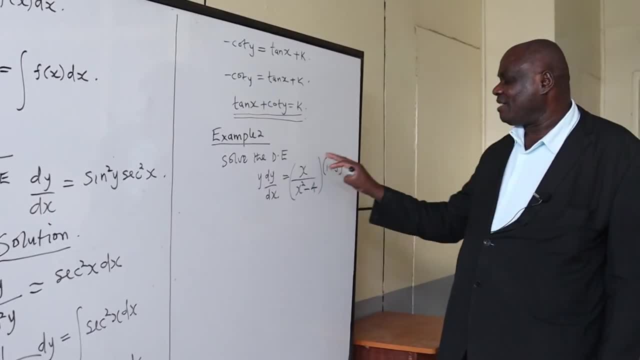 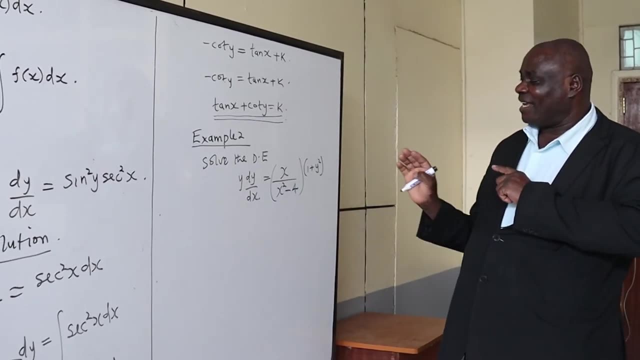 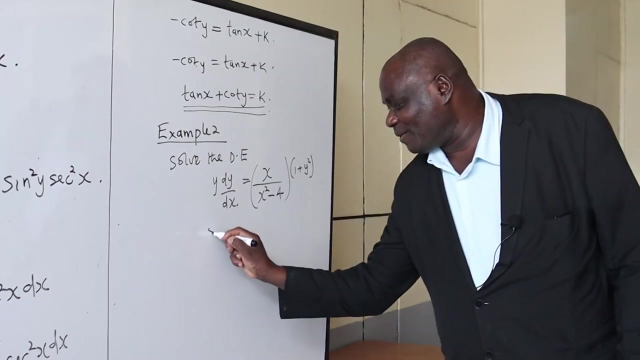 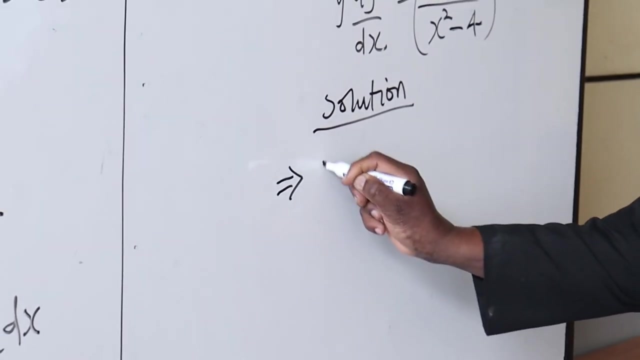 Into One Plus Y The Variables, Such A Way That We Functions Of Y Can Be Taken To Where We Have A D, Y And Functions. 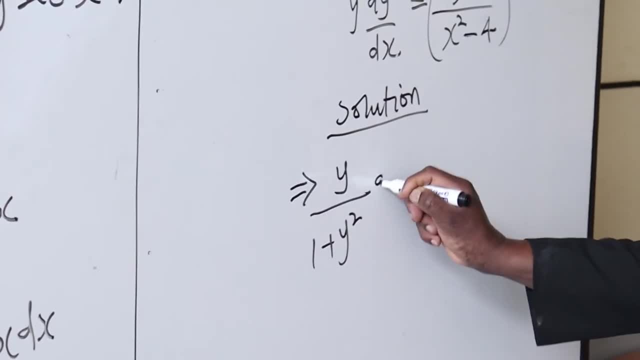 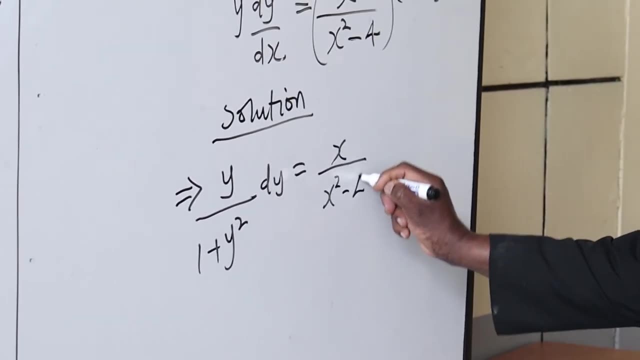 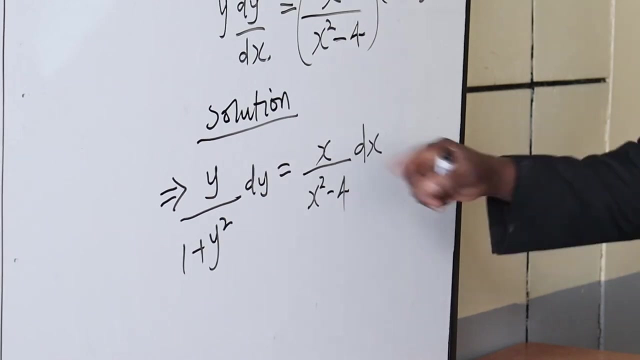 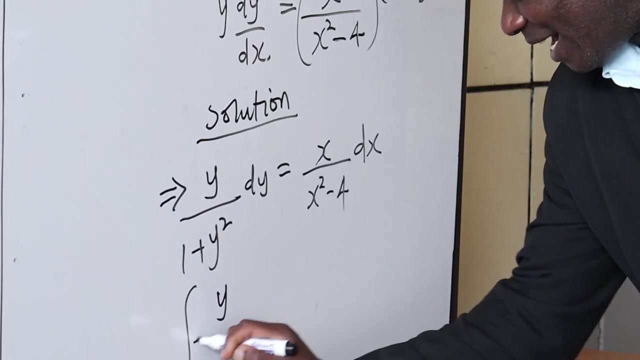 Of X Can Again Be Combined With X All Over X Square Minus Four D D X. After Separating The Variables, We Can See The: 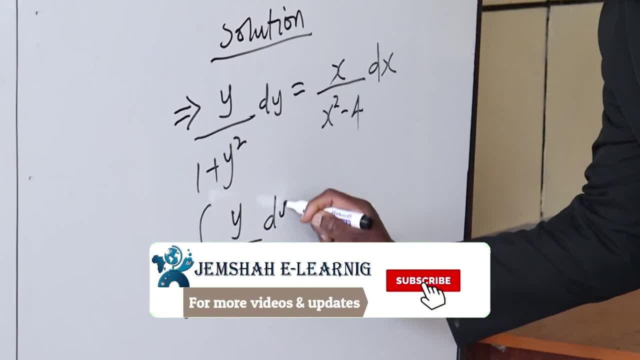 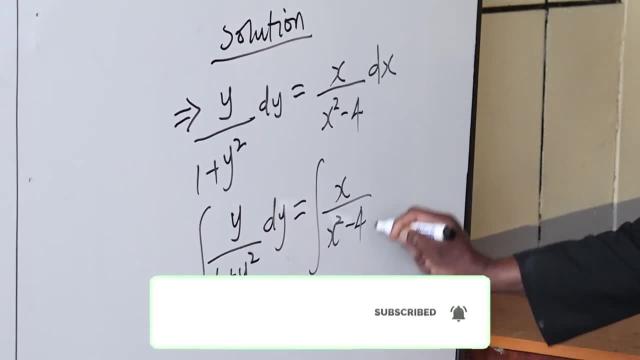 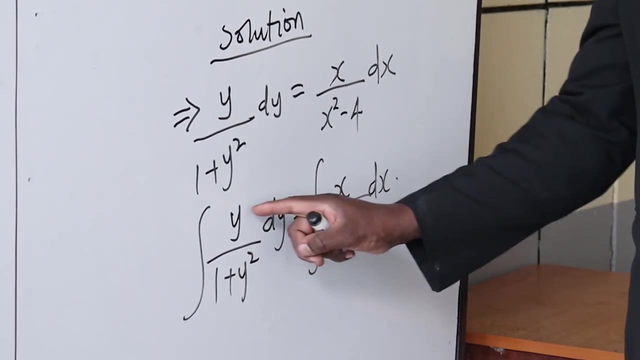 Variables Has Been Separated. The Variables Have Been Separated. Then We Have D X. Now Here We Have A Quotient, We Have A Quotient. 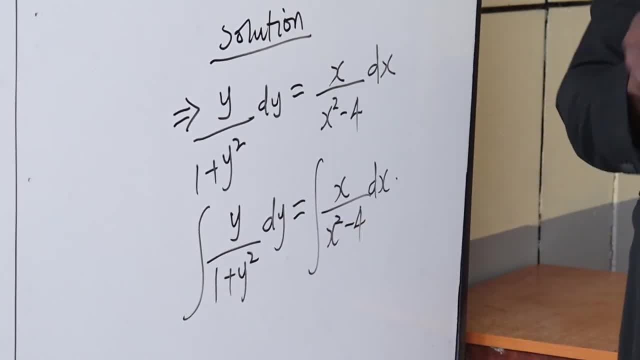 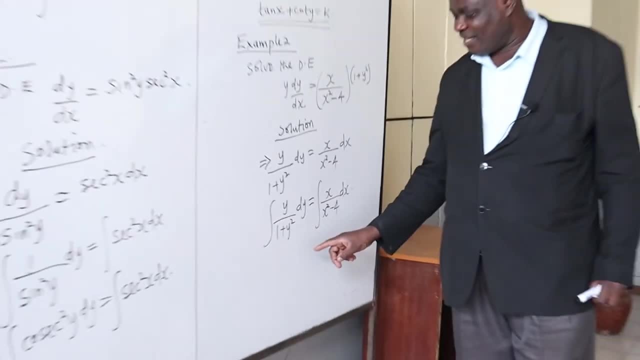 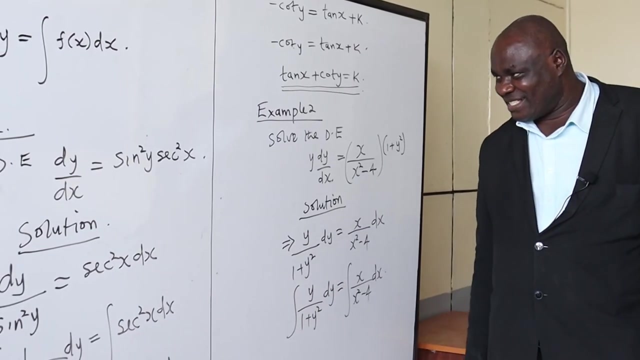 Y A Quotient Where We Have Numerator. Here We Have Y Denominator, Here We Have One Plus Y. So If We Have A Two, 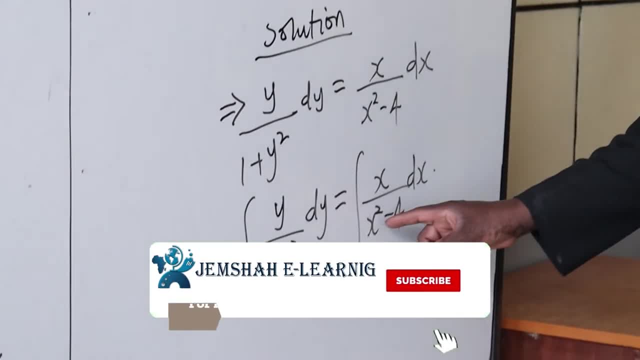 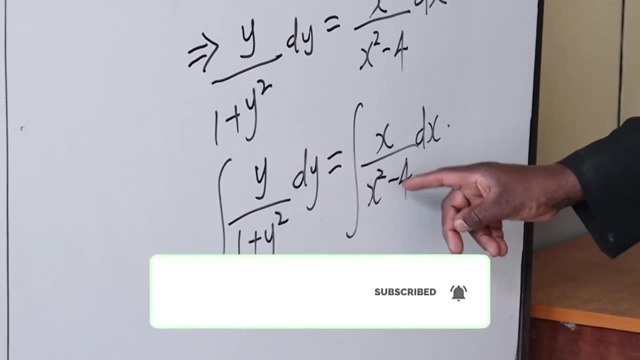 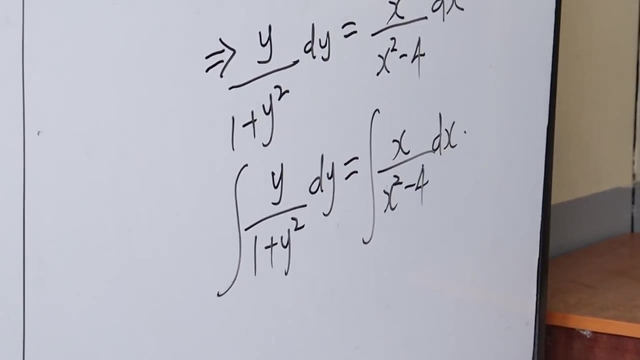 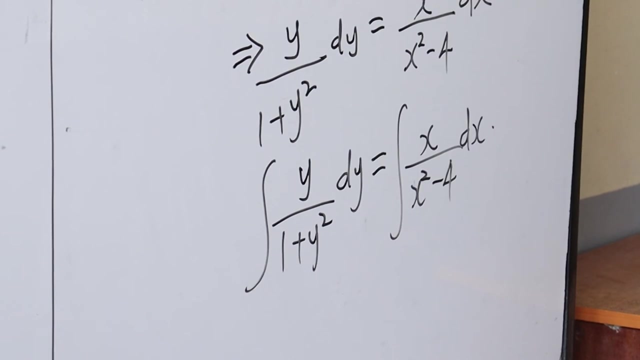 Up Here. Then We Can Be Able To Solve That Integral Easily And Also This One. We Have X All Over, X Away If You Multiply. 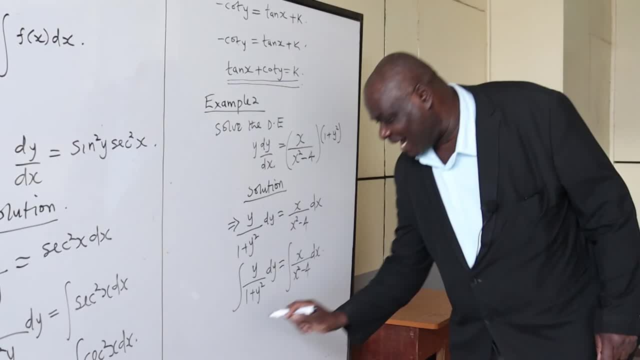 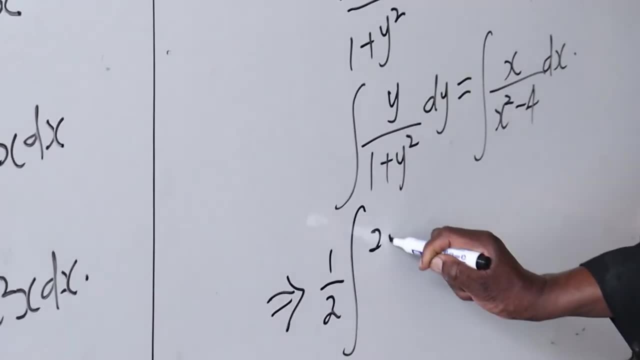 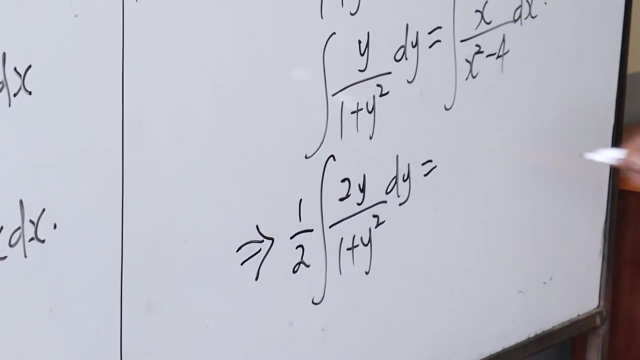 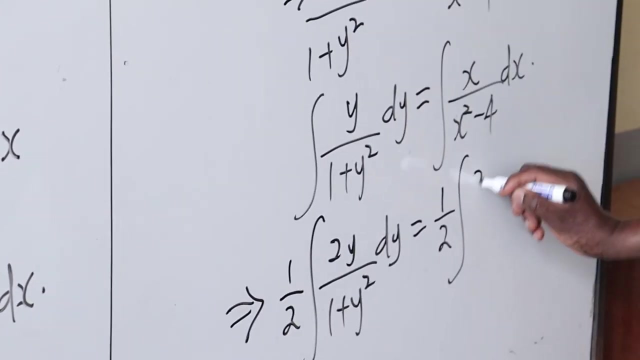 By A Constant, Then You Can Take It Away By Dividing By The Same Constant. That Is Now Here. We Have One Over Two, The 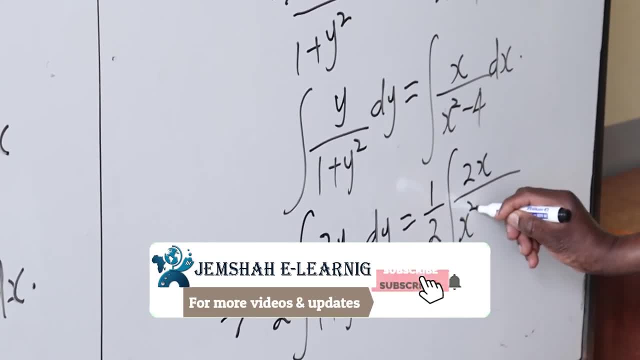 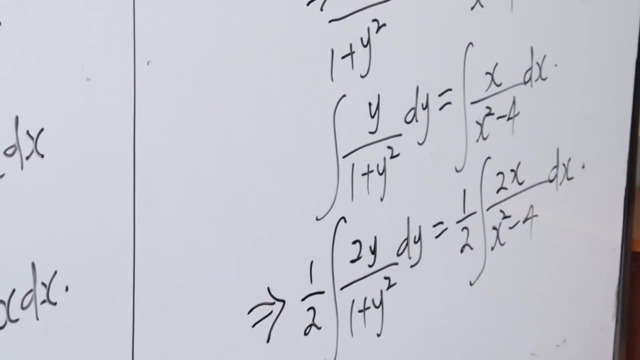 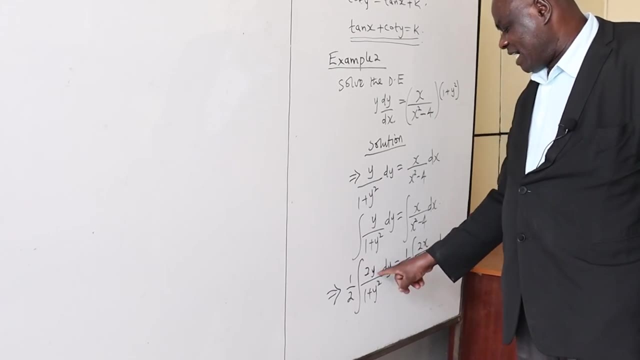 X All Over X Squared Minus Four. Now D X. Now, If The Numerator Is The Derivative Of The Denominator, When You Integrate. 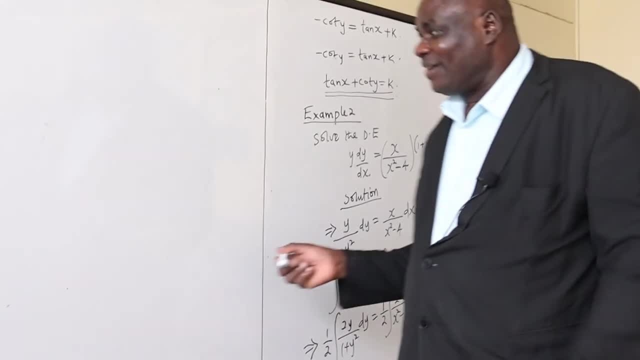 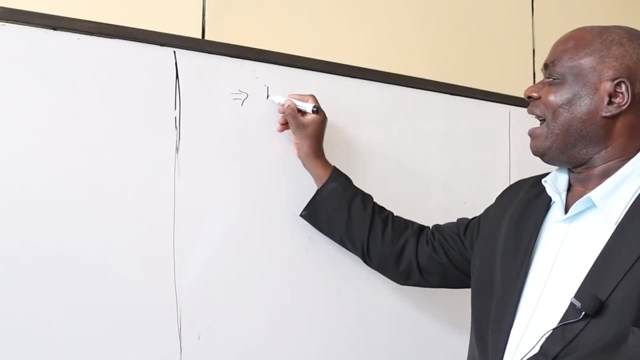 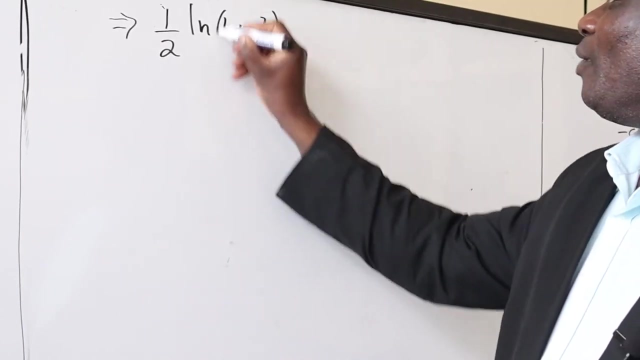 Such A Quotient, The Answer Becomes L. So This Implies A Half L N, A Half L N Of One Plus Y Square Will. 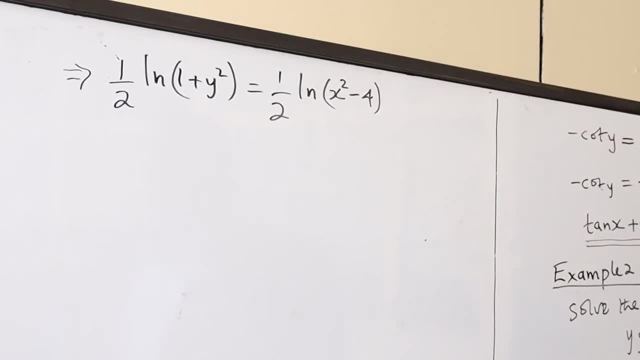 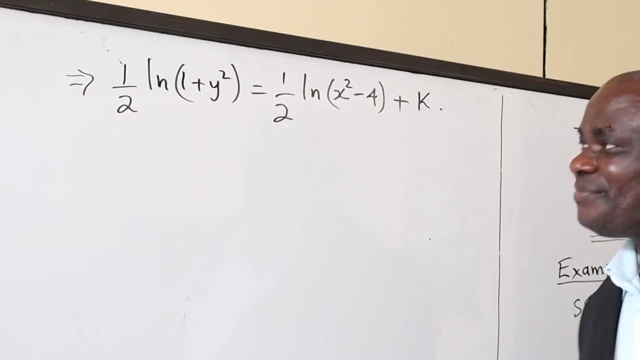 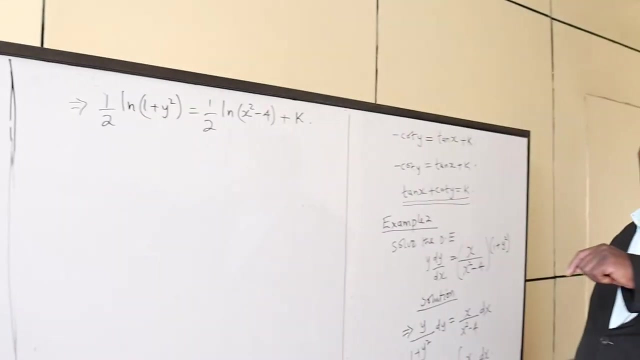 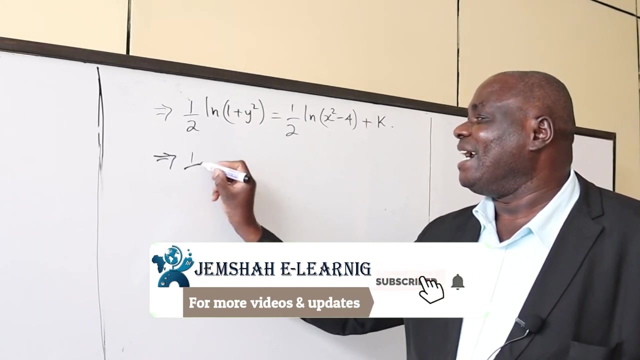 Be Equal To A Half. L N Of X Squared Minus Four Plus L N Of One Plus Y Square Is Equals To A Half. 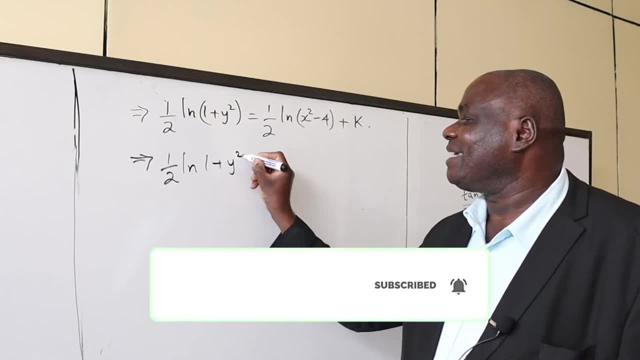 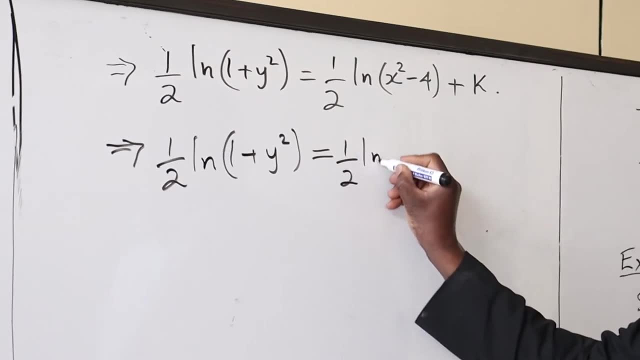 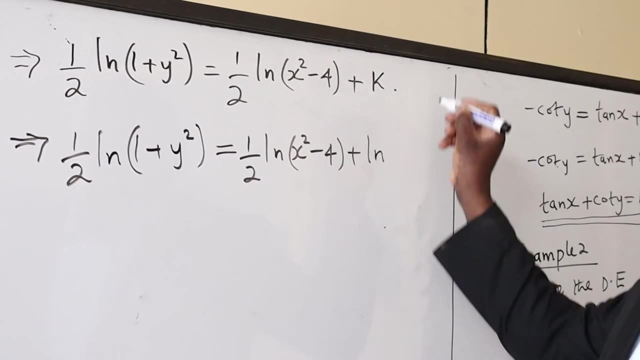 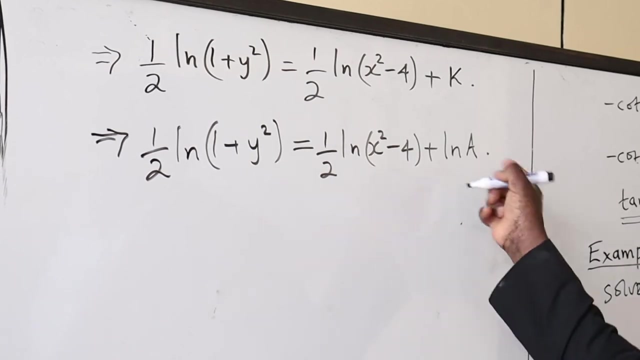 L N Of X Square Minus Four Plus L N Of X Square Minus Four Plus L N Of Another Constant. We Can Call It: 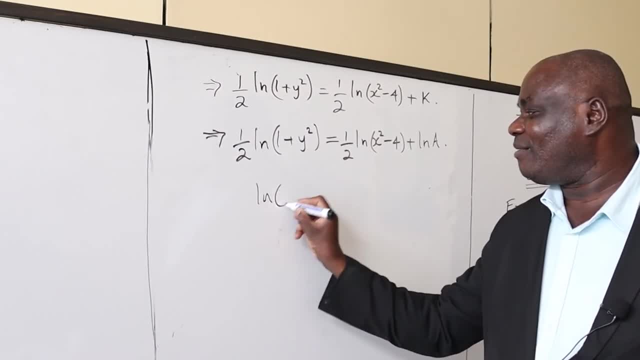 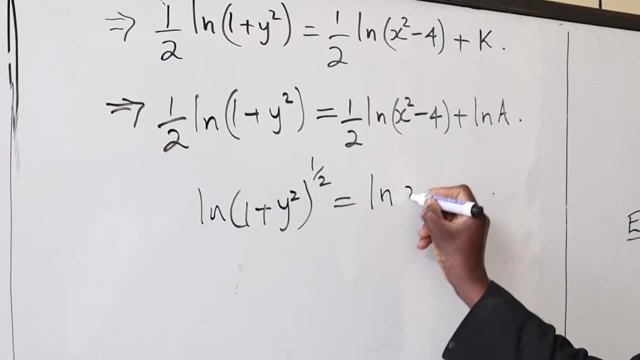 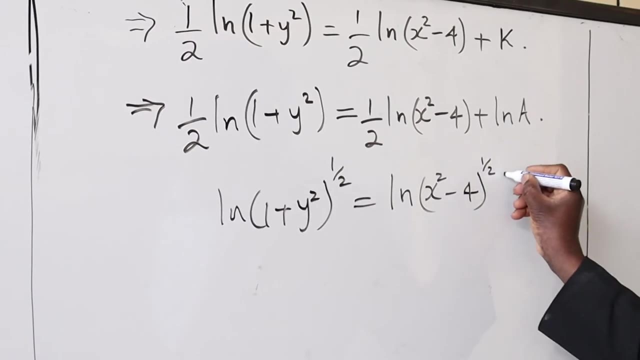 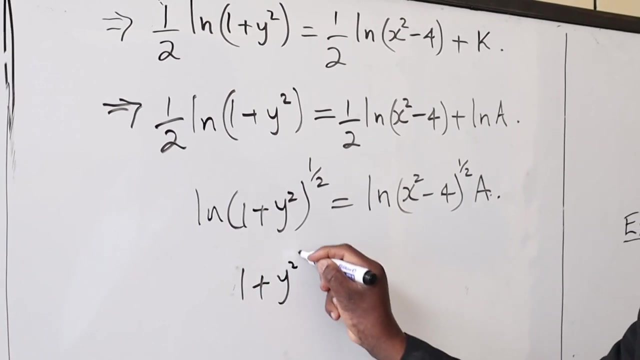 Constant A. Now We Can Combine This Through Loss Of Logarithms. This Will Be Equal To L? N Of One Line A, Which Gives Us: 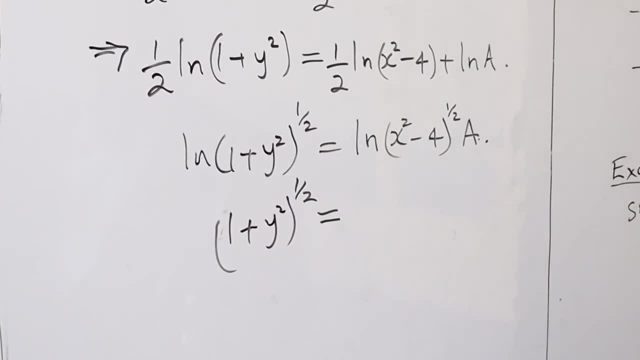 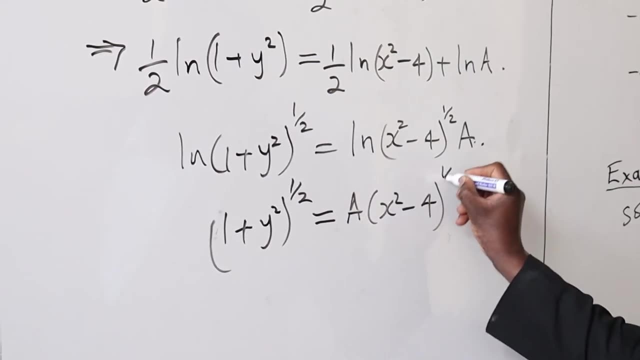 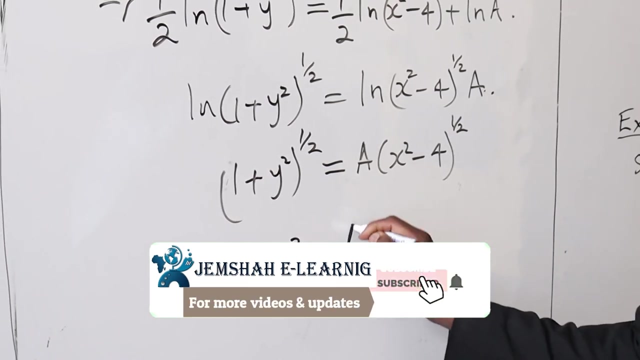 One Plus Y Square, Then Is To Power Half Will Be Equal To A Into X Square Minus Four Is To Power Half. Now A. 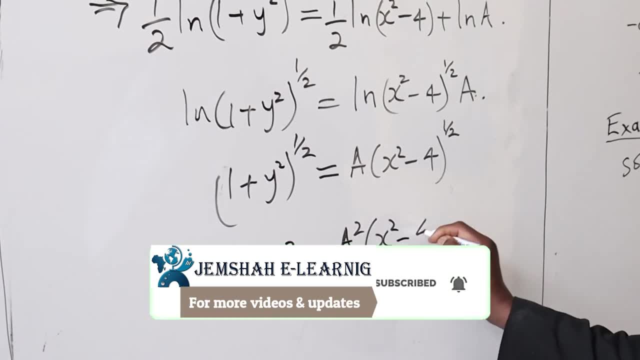 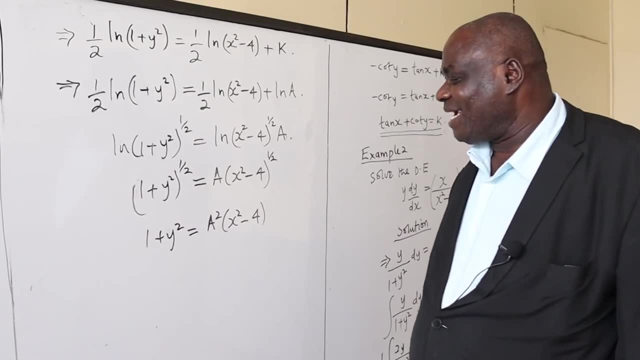 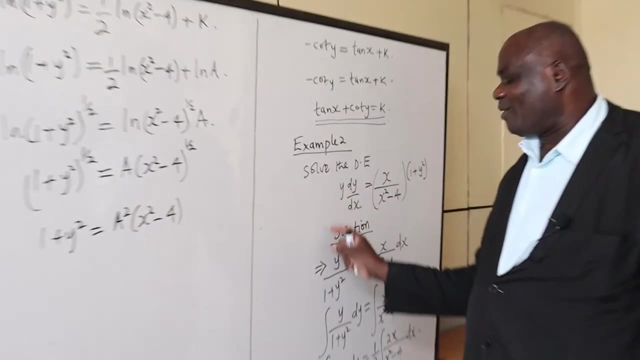 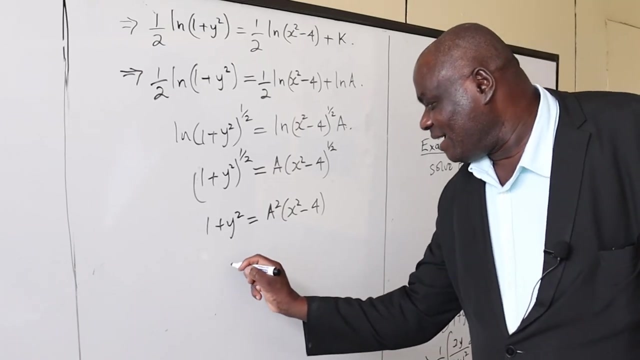 Square Into X Square Minus One. But A Square Is Just Another Constant. We Can Even Call It B. These Are Just A Bit Constant. 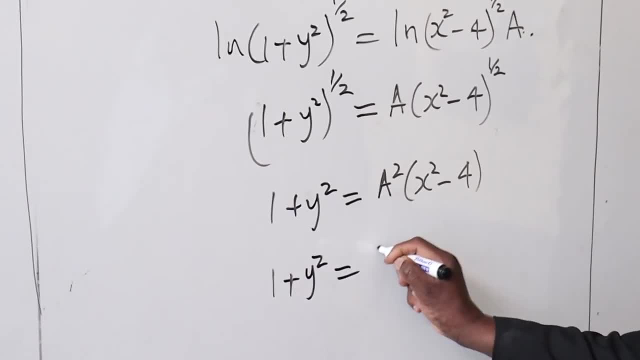 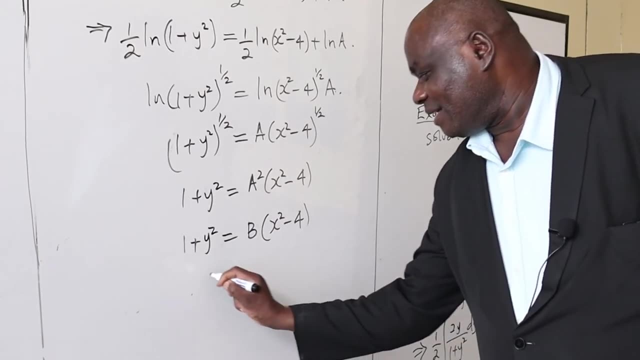 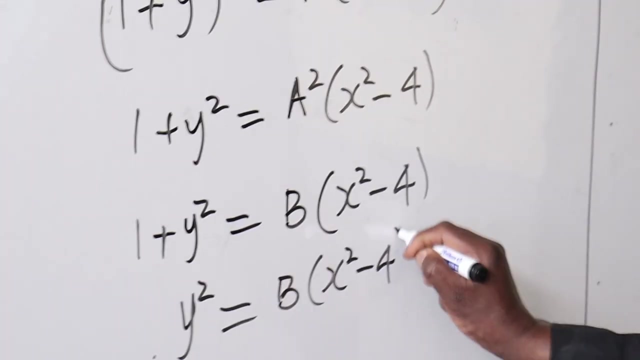 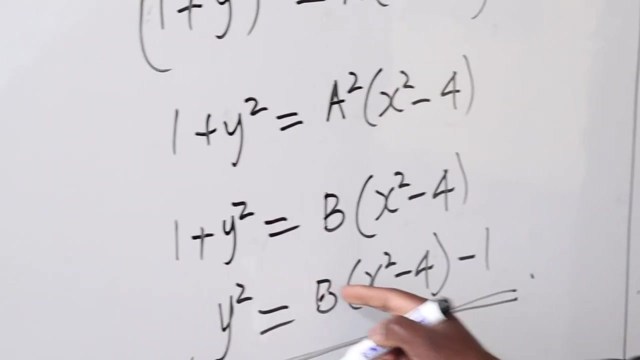 Because We Didn Have B B Stands In For A Square To X Square Minus Four. Therefore, Y Square Will Be Equal To B Into. 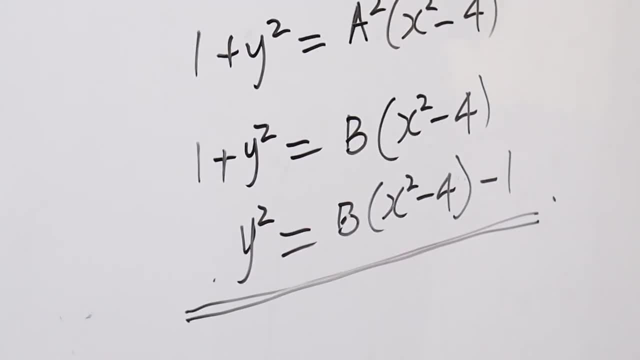 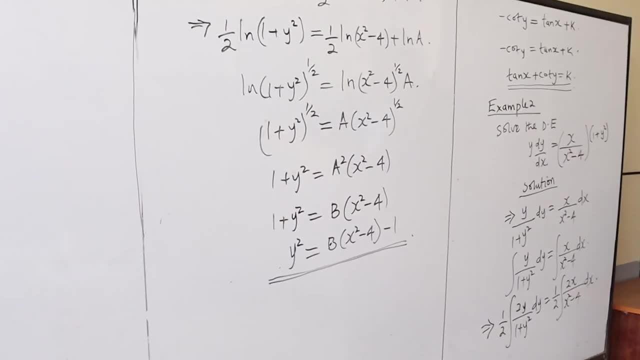 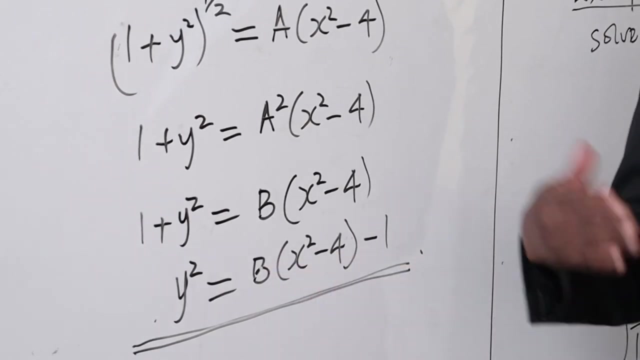 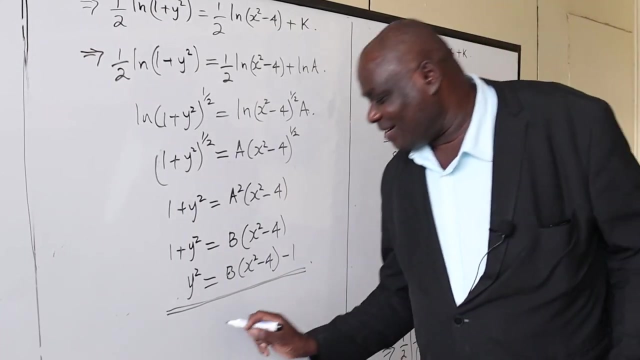 X Square: Minus Four. This One Minus One. Now We Can Get The Value Of B. Now We Can Get The Value Of B If. 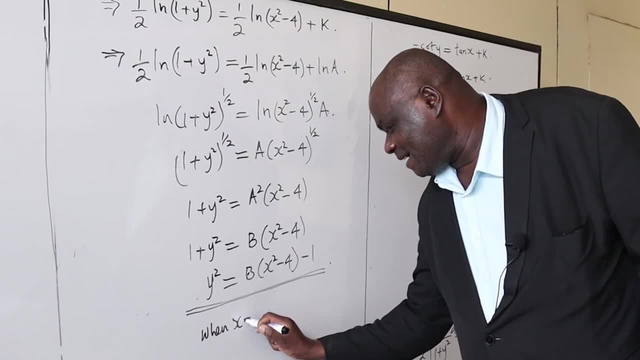 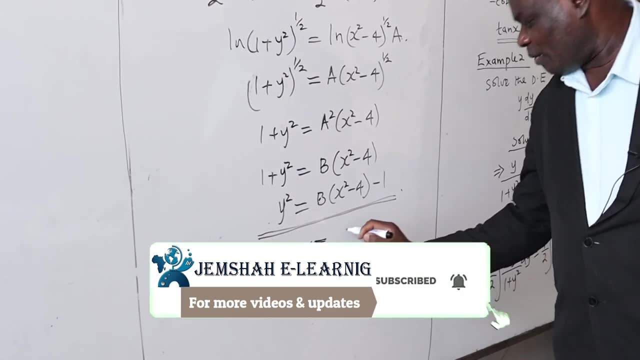 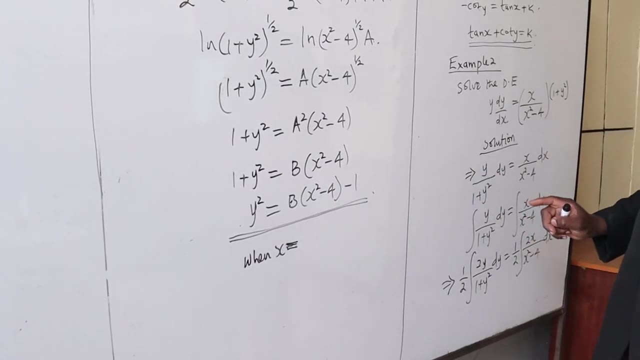 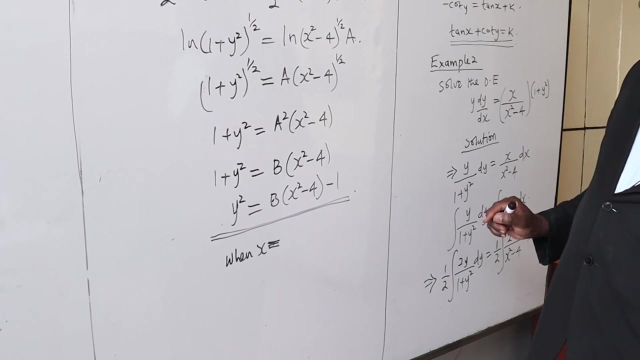 Some Conditions Were Given For Example. Now, If We Can Be Told When You, If We Imagine That We're In A Square, Also To Go. 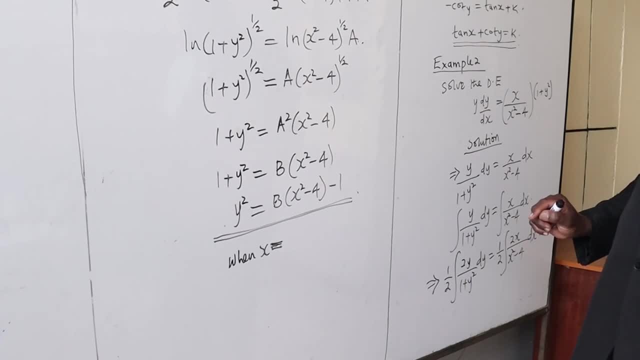 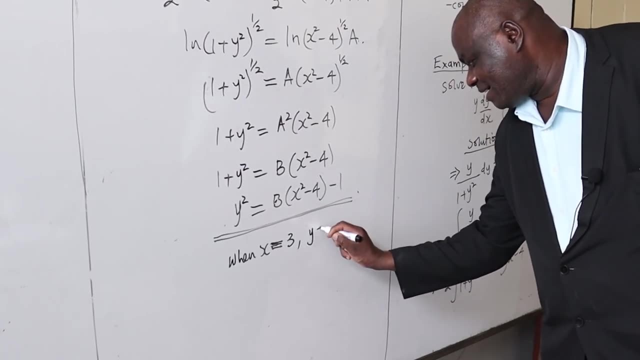 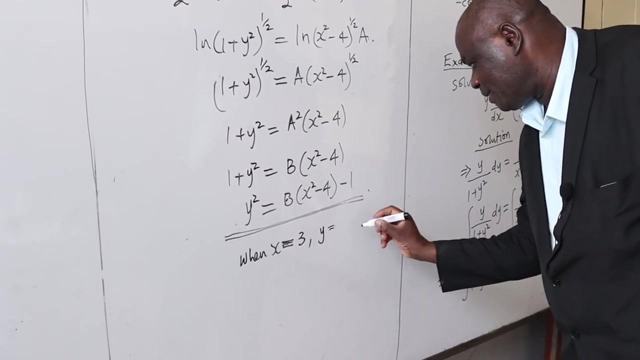 Together. Now For One, Each, All, All To The Appearance, To The Author Of Appearances. And Same Now. And x is equal to 3,, y is equal to 2.. 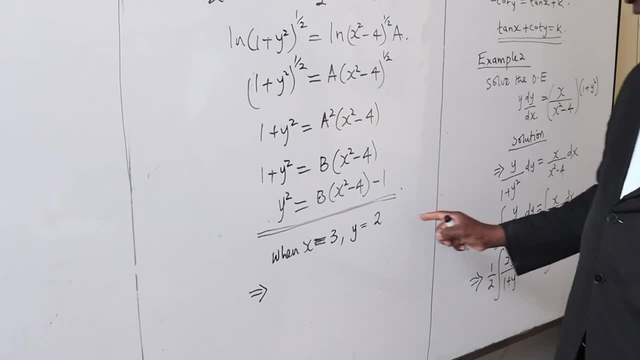 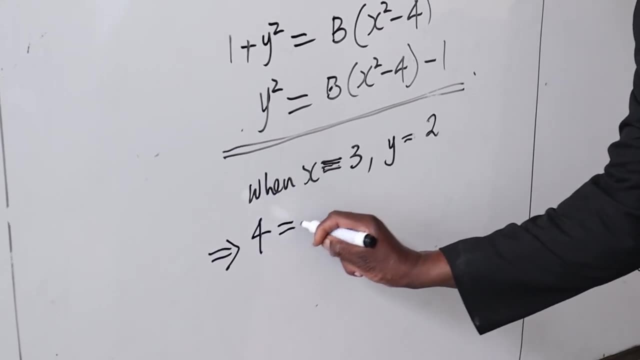 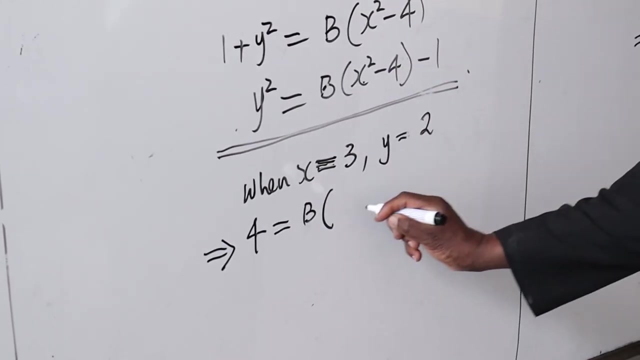 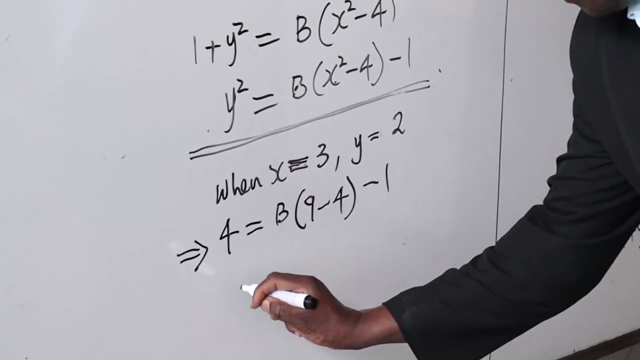 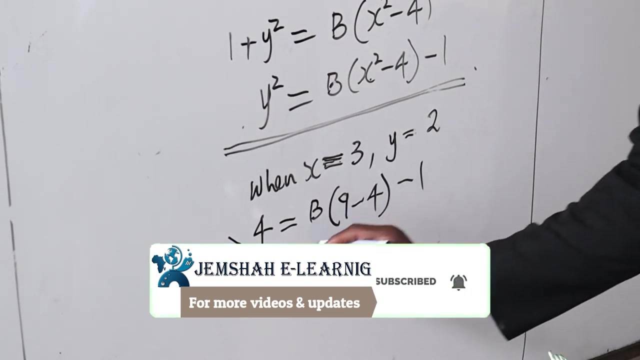 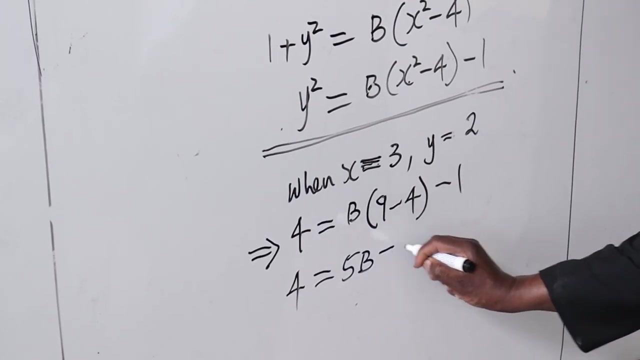 So this implies. this implies: whether it's y, we insert 2,, so this one will be 4, is equal to b into x squared. our x squared will now be 9, minus 4, then minus 1.. So this implies: this implies 4 is equal to 5b minus 1.. 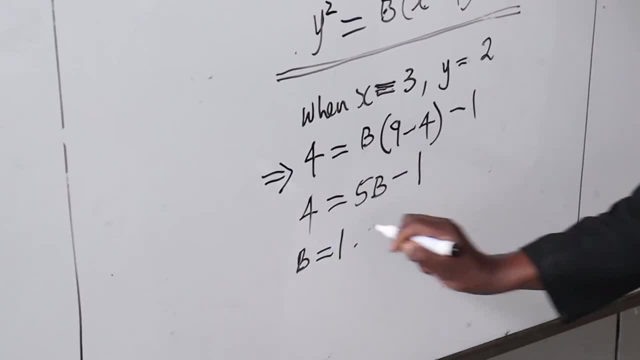 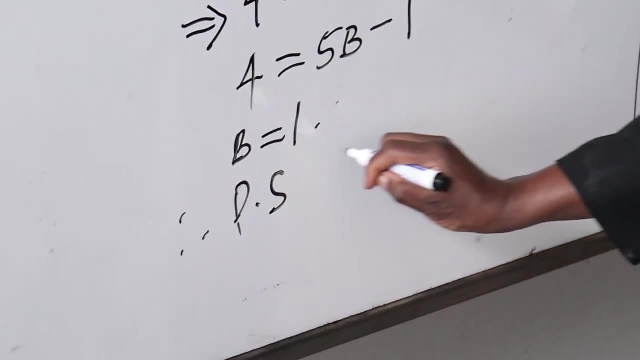 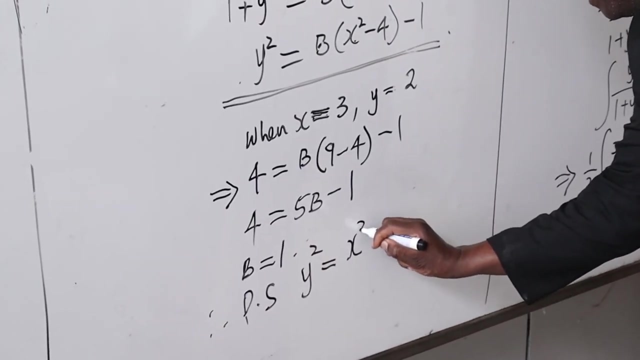 So b is equal to 1, b is equal to 1.. Therefore, particular solution. now we will read: y squared is equal to 1.. Okay, 2.. y squared is equals to x squared minus 5.. And that is the solution to the same differential. 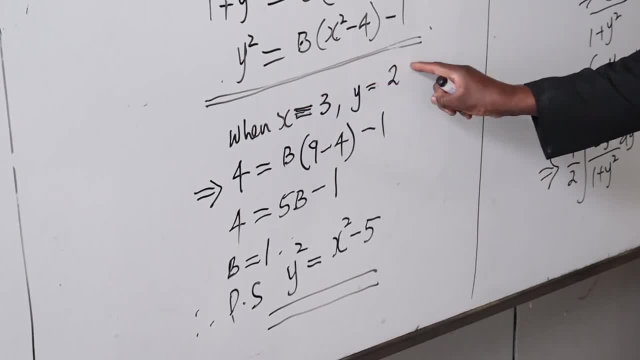 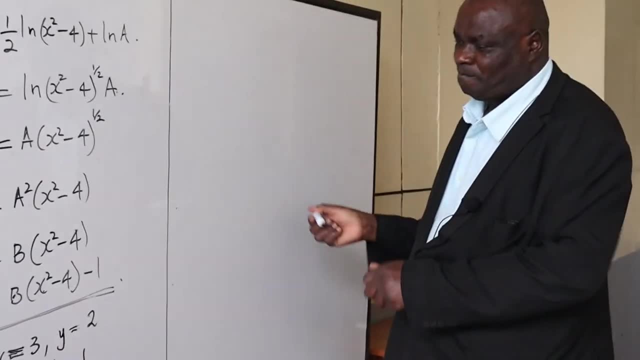 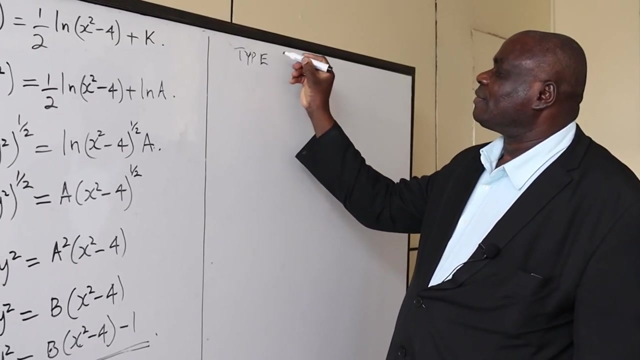 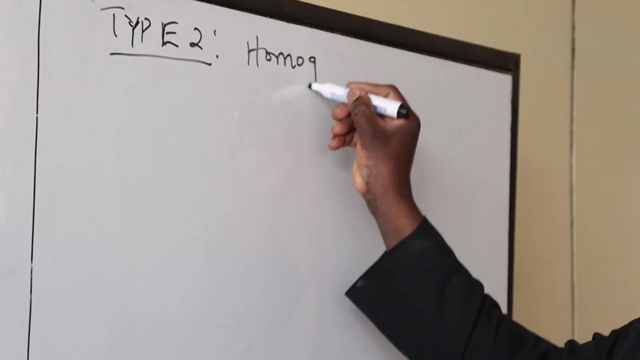 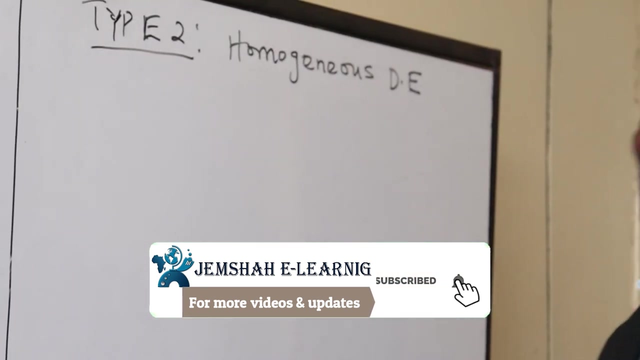 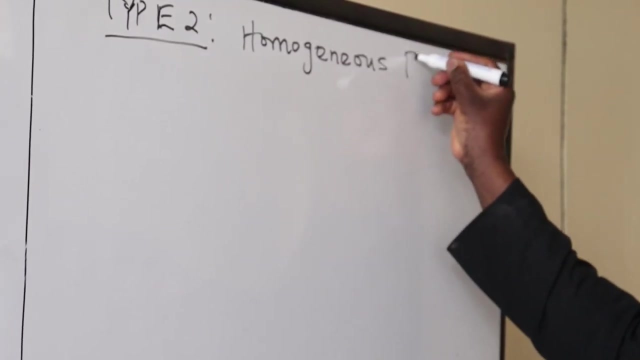 equation. when these are the boundary conditions that exist. Now move to type 2.. Type 2. Homogeneous- Homogeneous, Differential. Differential. Differential equation- First order: differential equation- First order: Differential. Homogeneous. First order D. 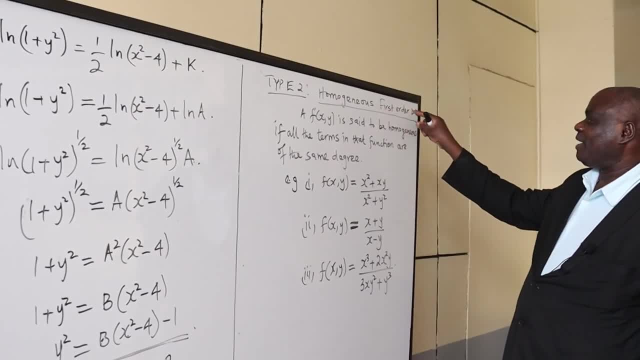 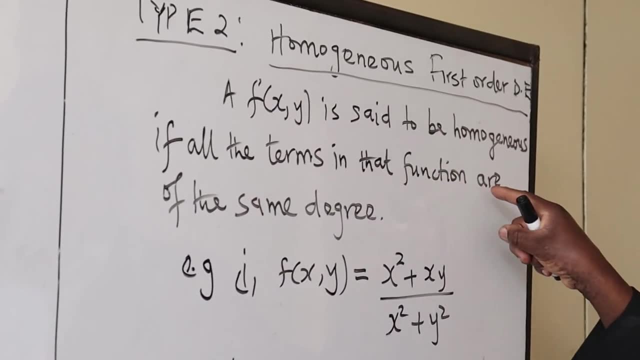 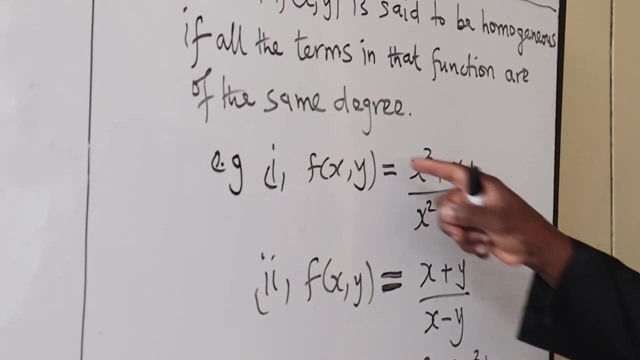 So now at type 2 we have homogenous, first order D. We say a function of x- y is said to be homogenous if all the terms in that particular function are of the same degree. Now we have a function of x- y, which is this one: X squared. 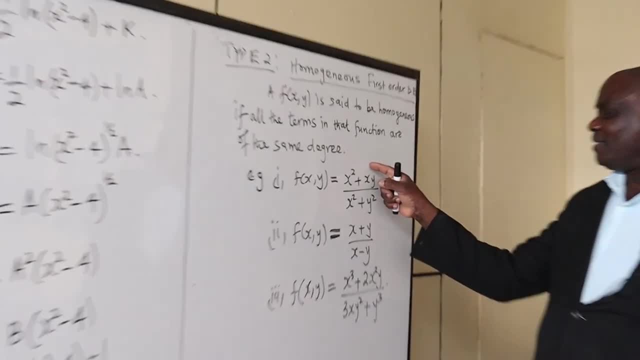 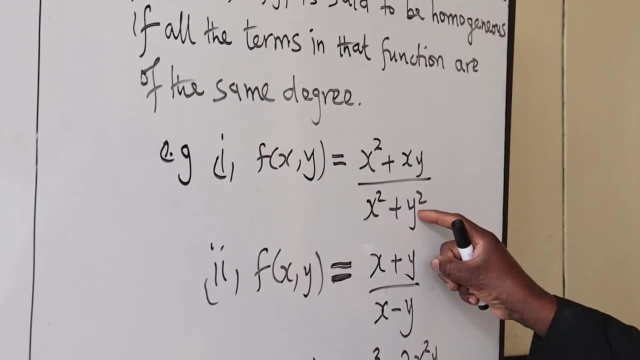 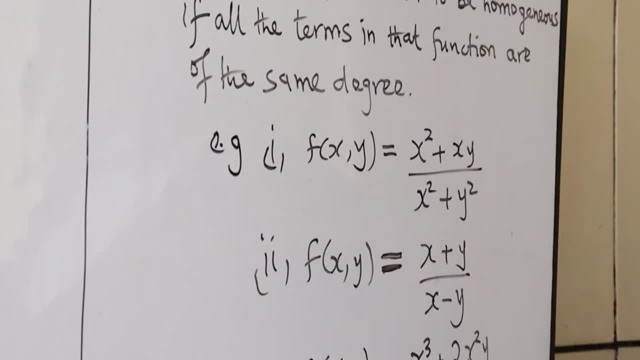 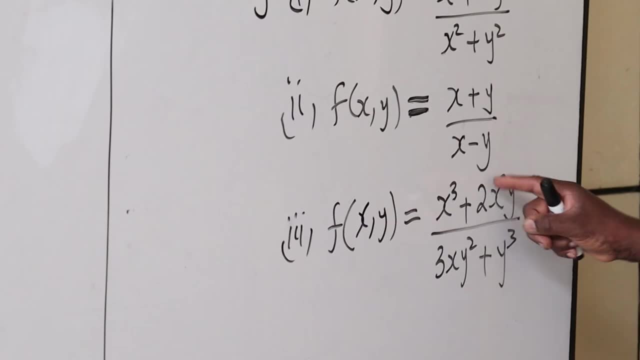 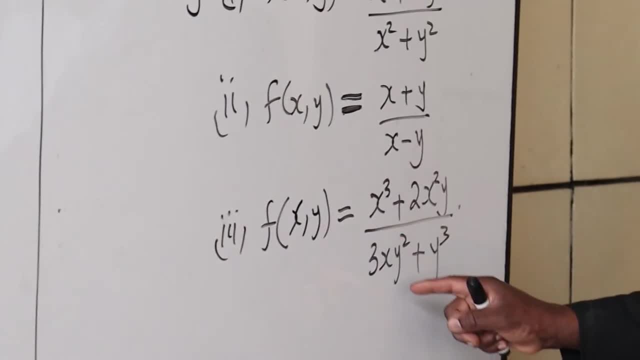 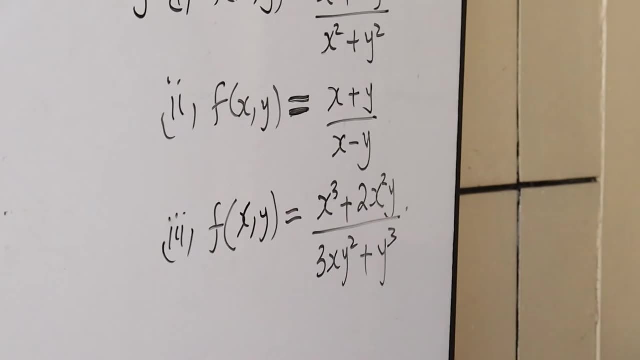 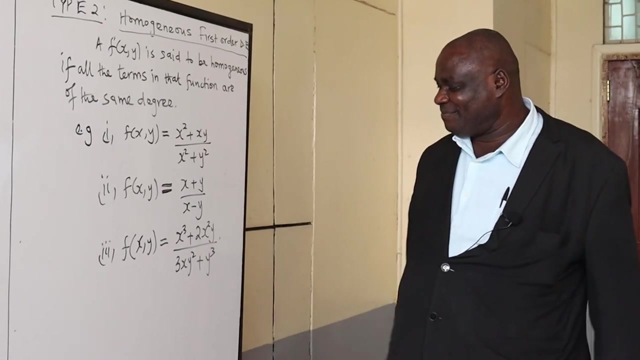 plus 2, 3.. So this one degree, 0.. X power 1, y power 2, we get 1 plus 2, we get 3.. This is y power 3.. So all are of the same degree. Now, if all are of the same degree, this is: 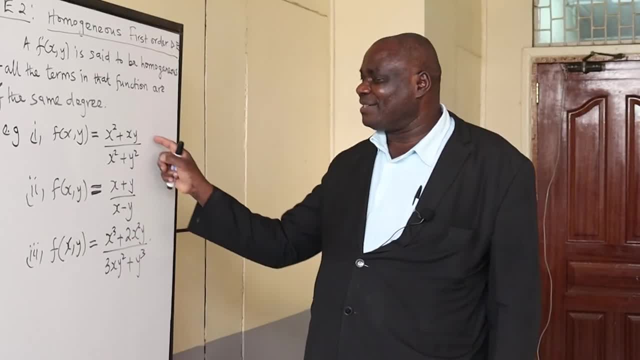 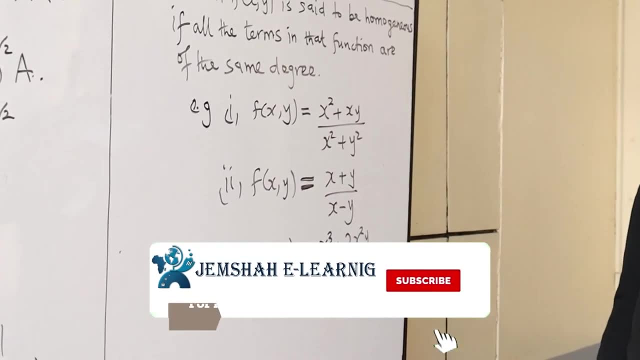 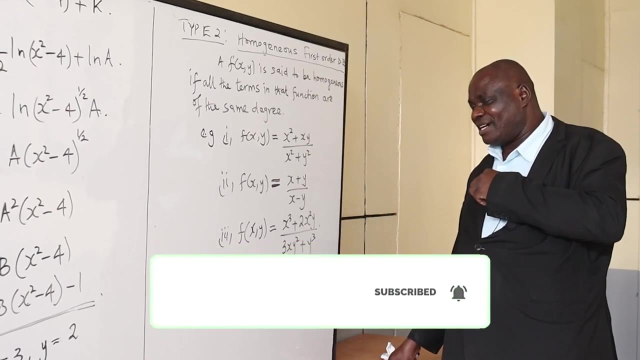 a homogenous function. This is also a homogenous function. That is also a homogenous function. And if we have a first order differential equation that we cannot be able to separate the variables And those within the function, we can see there is a homogenous function. 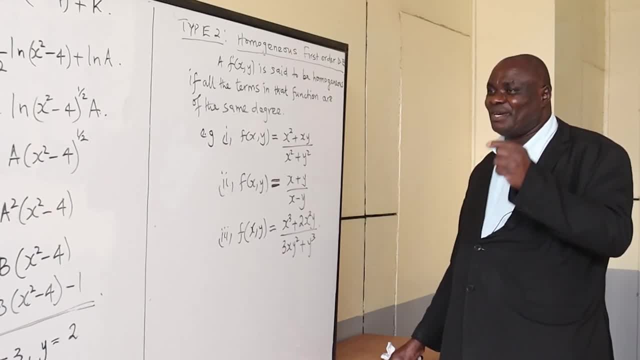 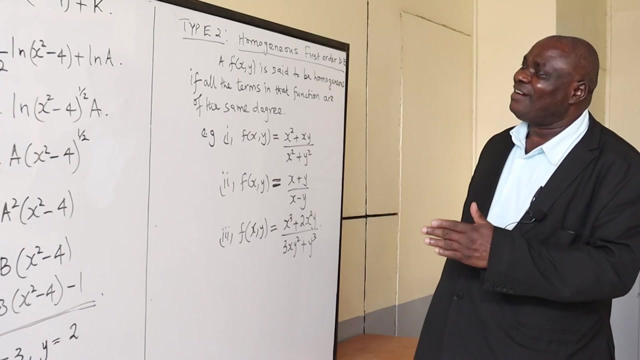 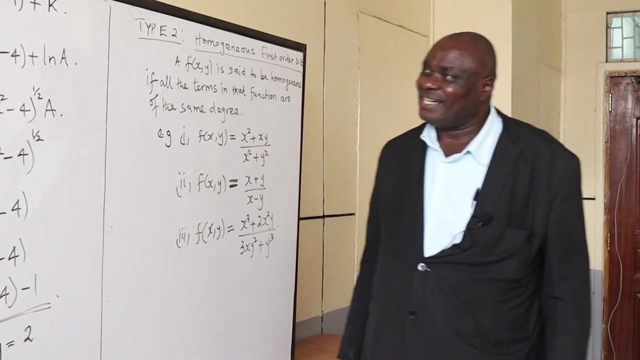 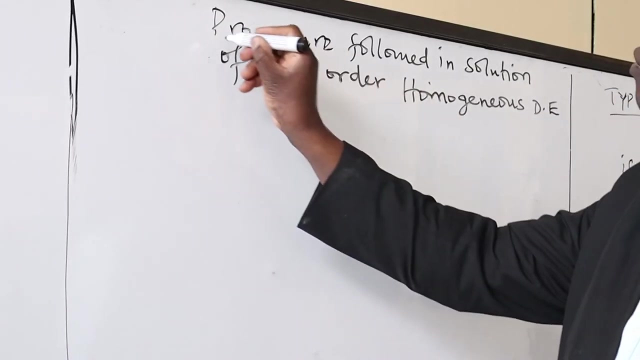 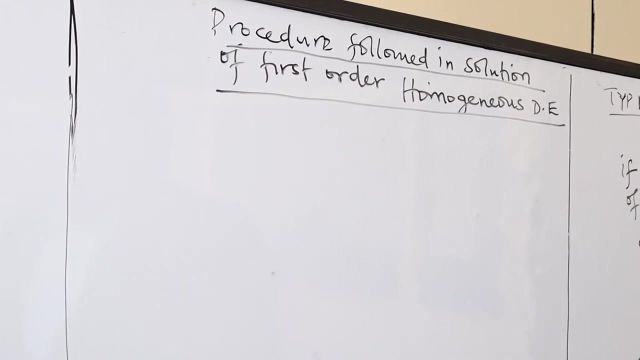 Then we can solve it using the procedure of solving homogenous first order DE. Now the steps to be followed or the procedure for solving a homogenous first order differential equation is stated as shown below. The procedure to be followed in a solution of first order homogenous differential equation. 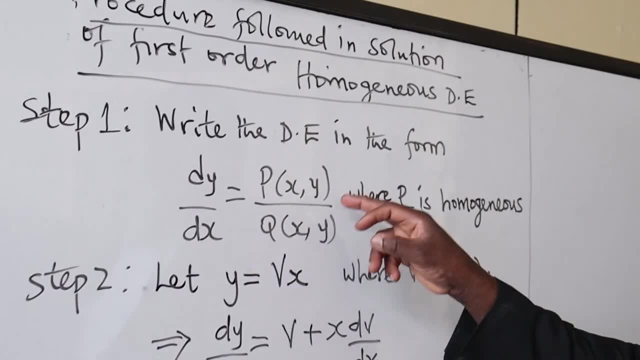 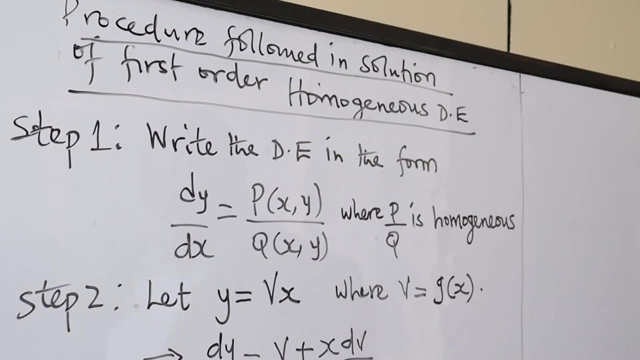 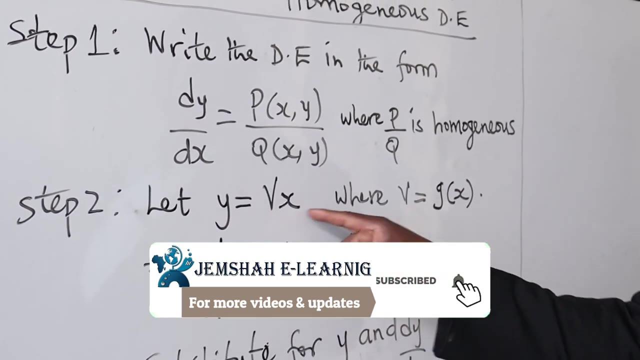 Step 1, write the DE in the form dy. dx is equal to pxy, all over q, xy, Where p over q is now homogenous. Step 2. We now let y to be equal to v times x, where v is another function of x, which we are calling. 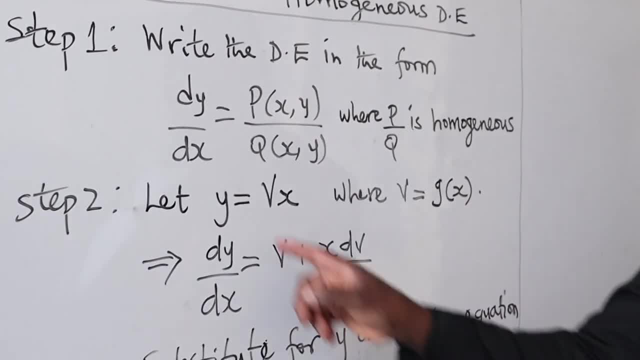 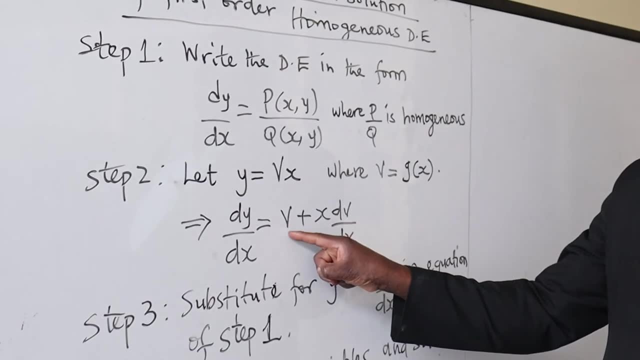 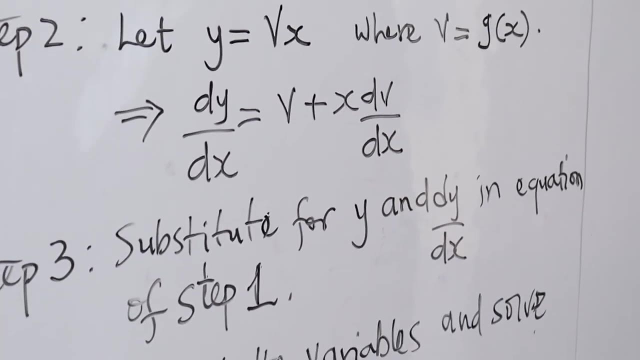 as g of x. This implies, if y is equal to vx, by using product rule of differentiation, dy dx will be equal to v plus x, dv dx, Step 3.. You substitute for y and dy dx in equation of x, Step 4.. 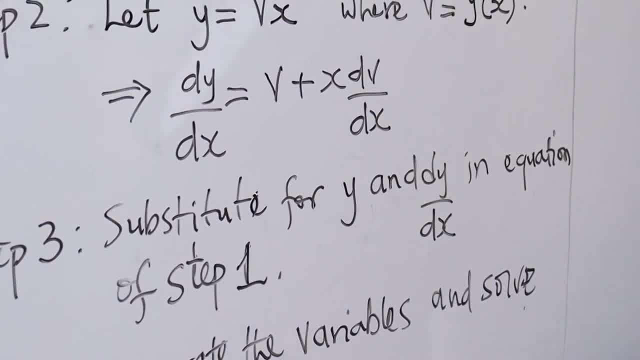 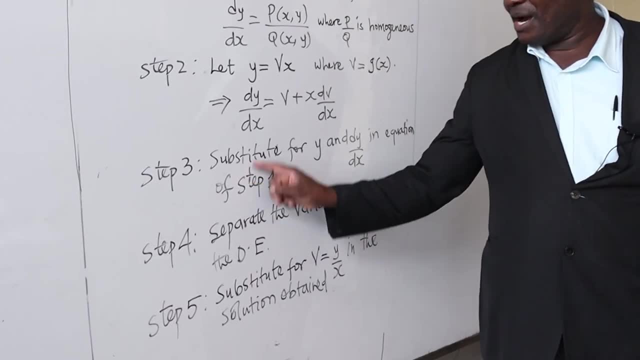 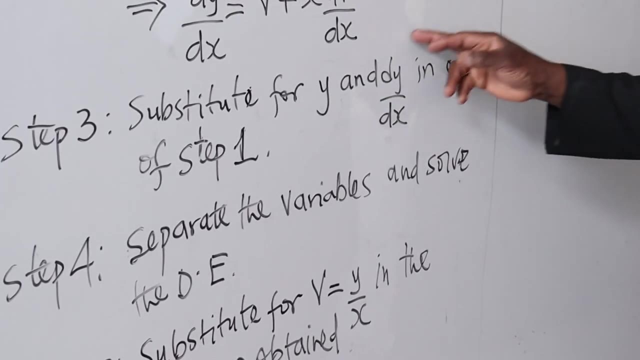 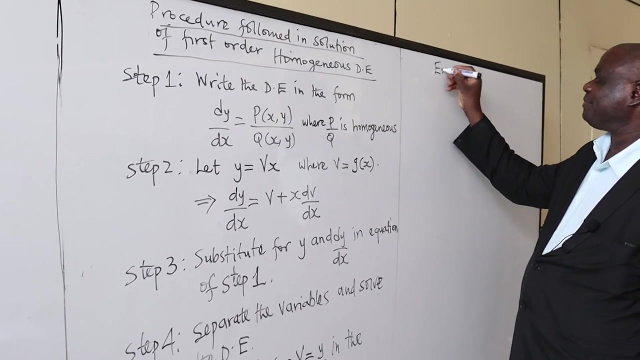 You substitute for y and dy dx in equation of step 1.. Step 1, which is this one: Now: after that, after substituting for y and dy dx, we will now do this. So let us have an example on first order. homogenous differential equation. 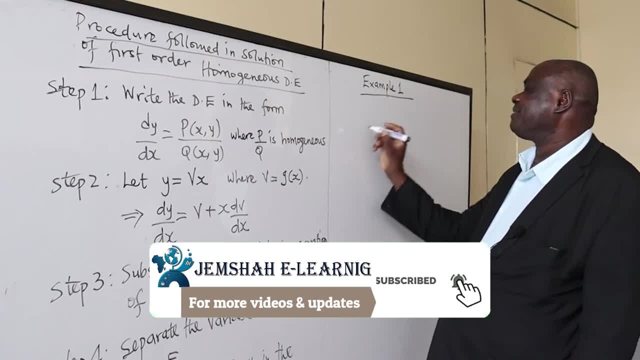 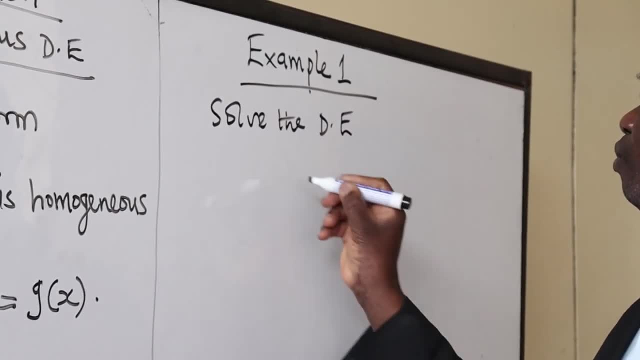 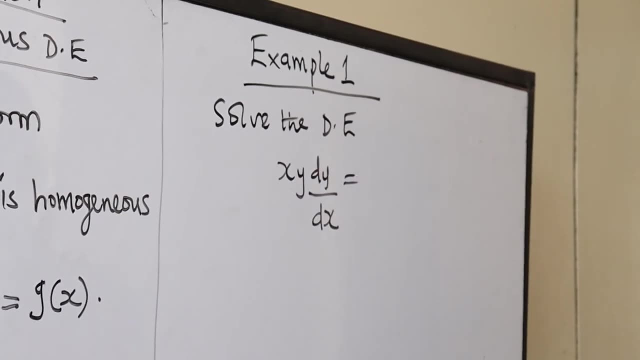 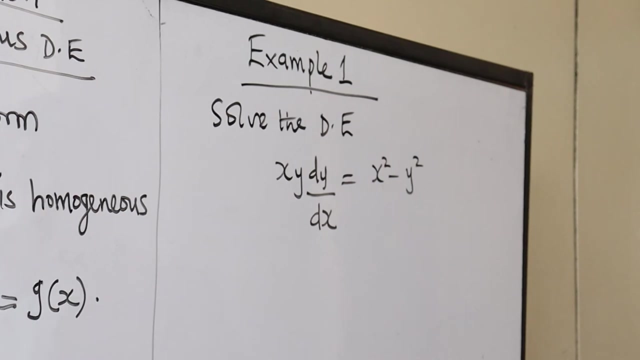 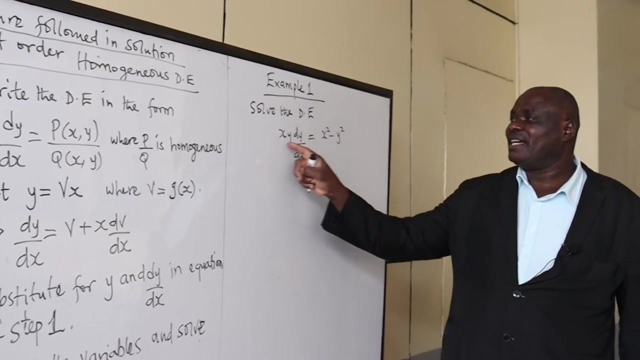 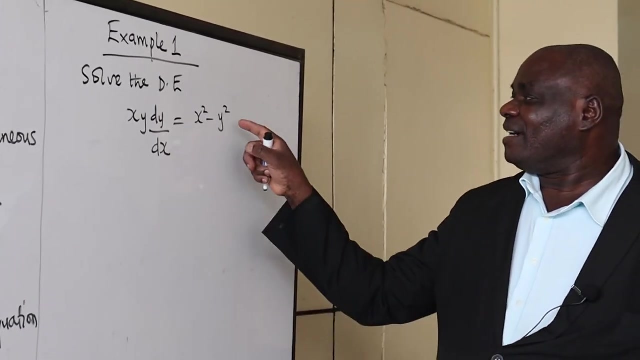 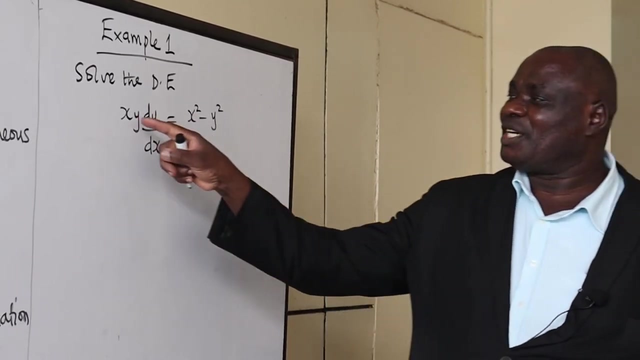 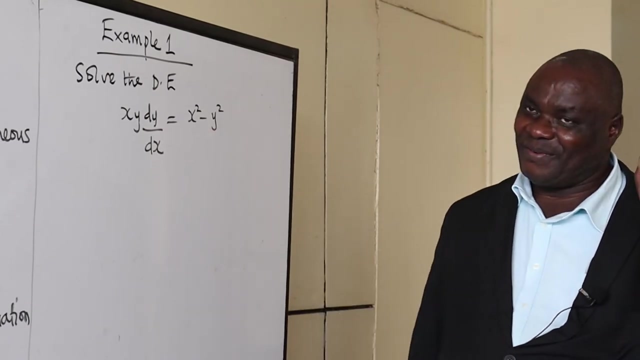 depression equation. Solve it by doing: xy divided by x is equal to x squared y squared. Solve it by doing: xy divided by x is equal to x squared minus y squared. Now, if we check x times, y is of degree 2.. x squared is of degree 2.. y squared is also of degree 2.. 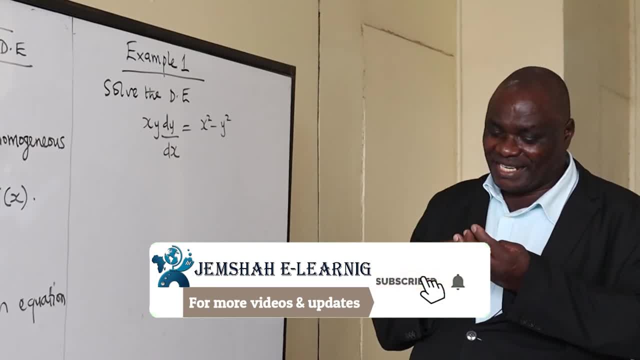 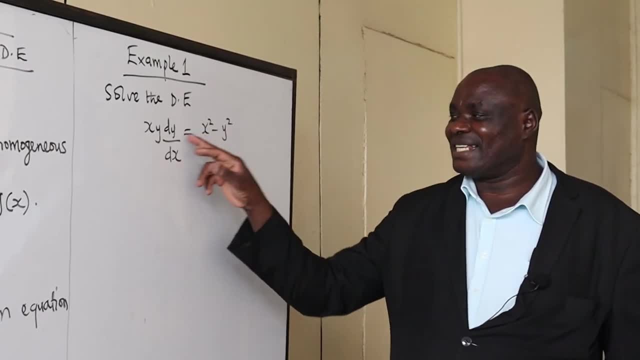 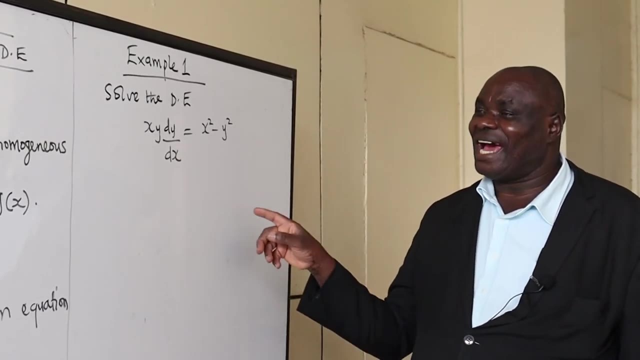 But even before we can see, those terms are of the same degree. But when we see these particular terms or these functions as they are stated here, we cannot be able to separate the variables. When we do so, it will take a long time to do it so tedious. 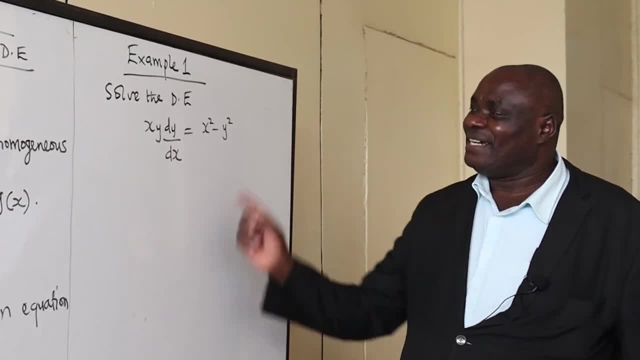 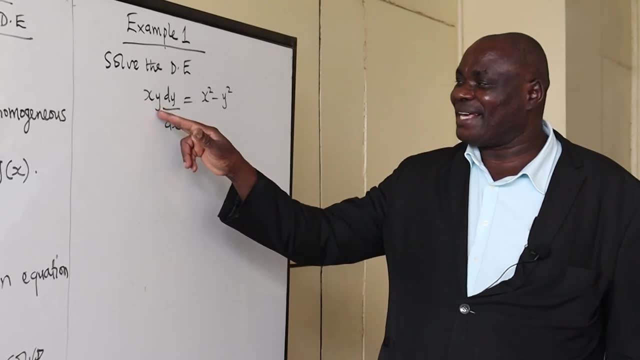 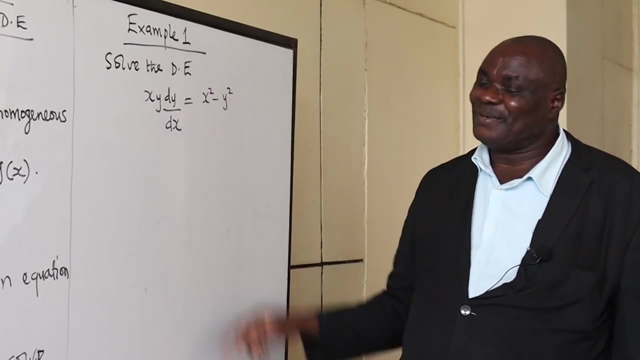 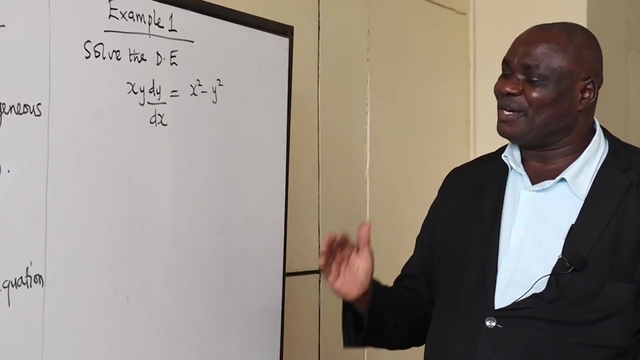 to enable us to separate y from x, And therefore the next step is to check whether the equation is homogeneous. And when we check now, degree 2, degree 2, degree 2. Then those terms are of the same degree And now we can now use the method of solving homogeneous differential equations. 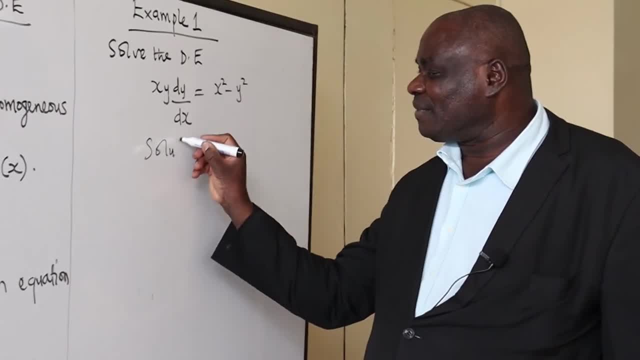 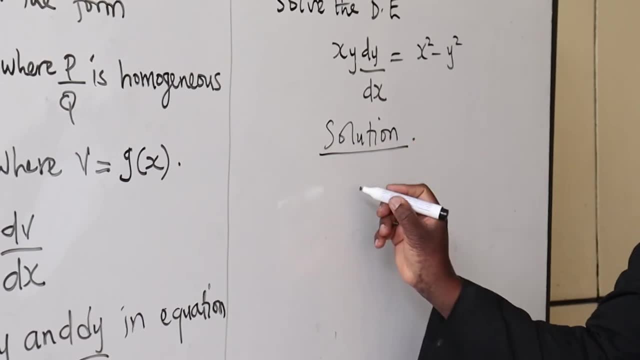 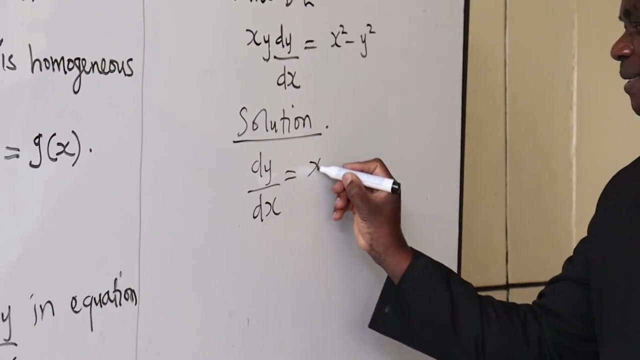 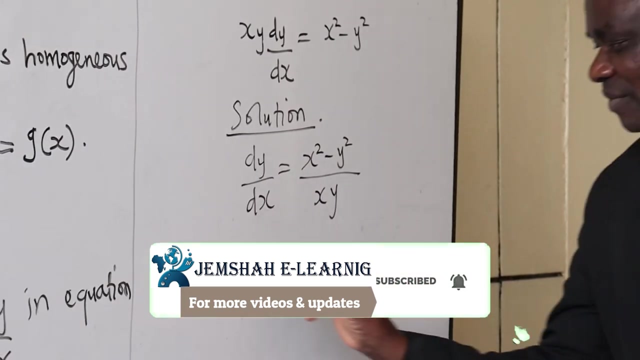 So in our solution, in our solution, in our solution, we can say from above: dy dx, and we've seen explicitly that this will be equal to x squared minus y squared, All over xy. From here we say: let y be equal to v times x. 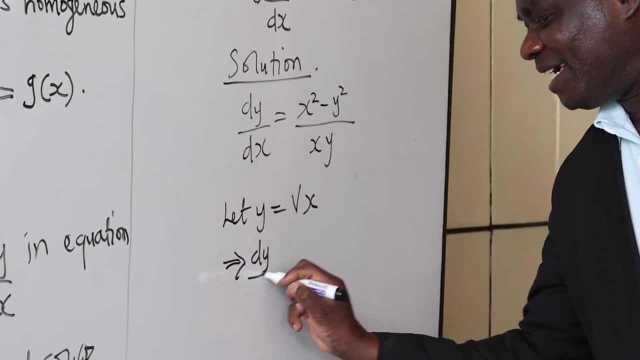 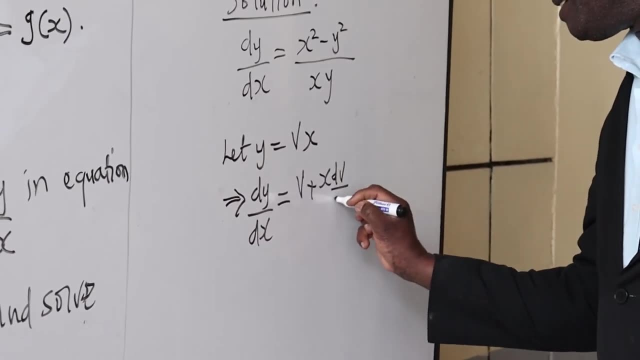 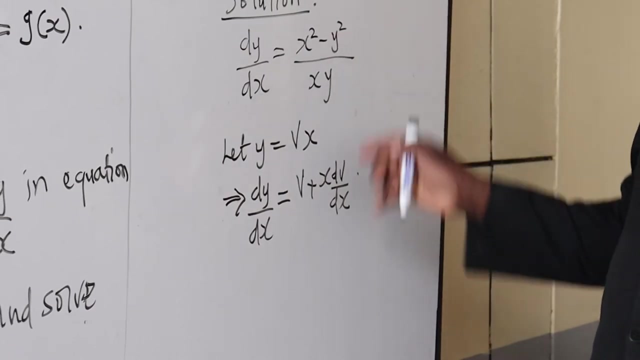 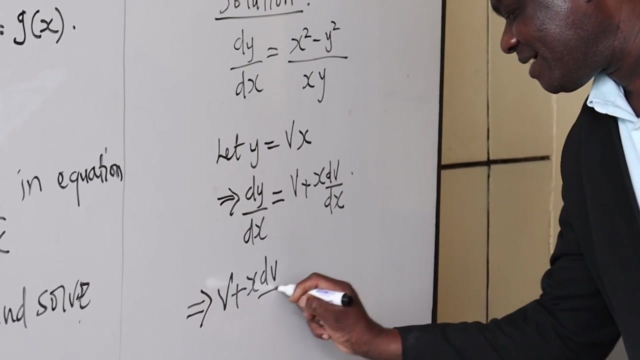 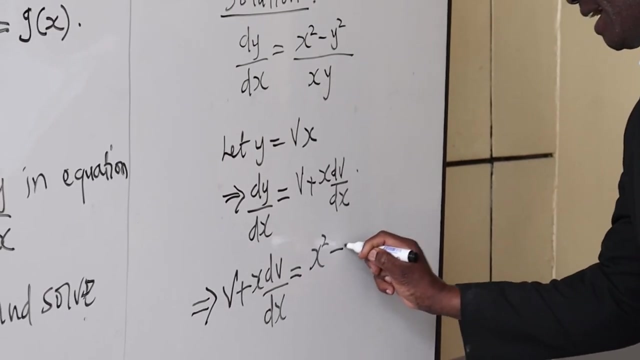 v times x. This implies what dy dx? This equals to v plus x dv dx. Now when we substitute into this first equation, we say this implies what v plus x dv dx? v plus x dv dx will be equal to x squared minus v squared. 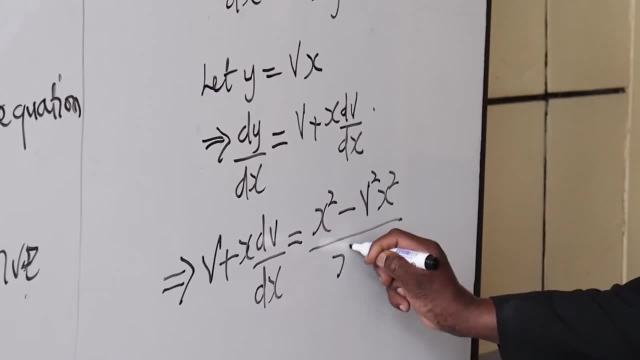 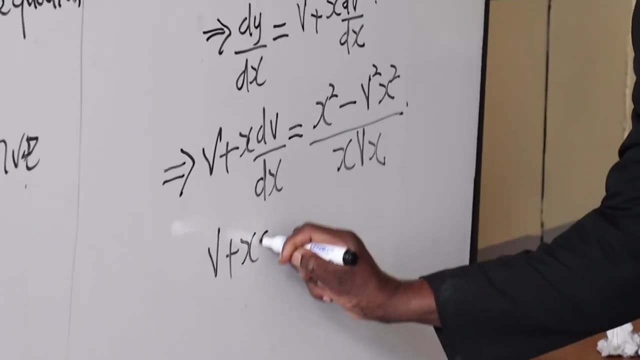 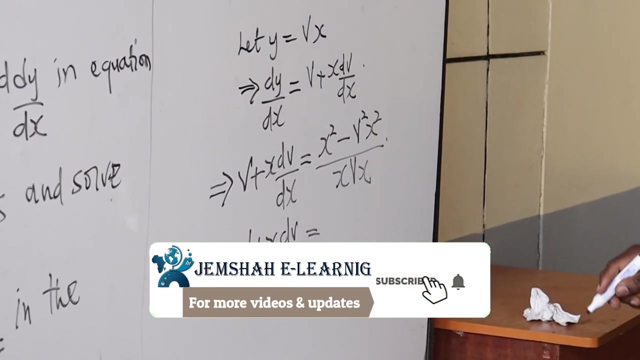 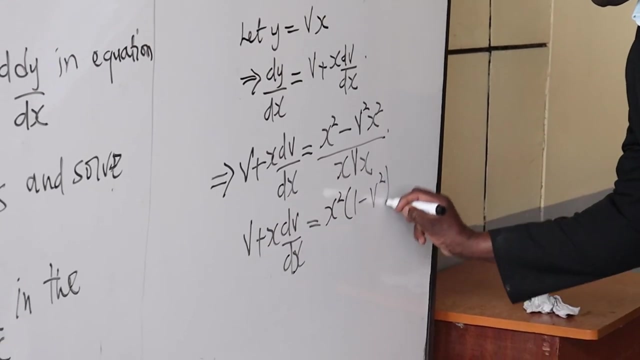 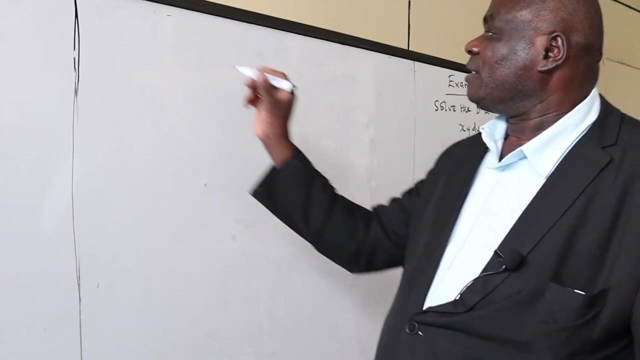 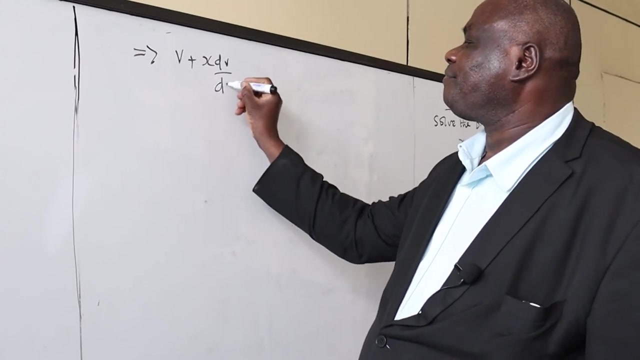 x squared all over x multiplying vx. So v plus x dv dx will be equal to: as you can see, this will be x squared into 1 minus v squared All over x squared v. So this implies that v plus x dv dx. 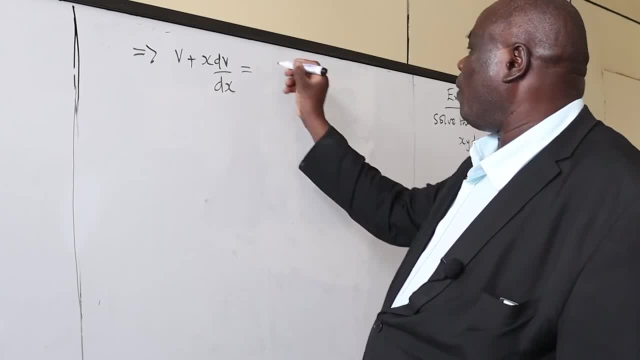 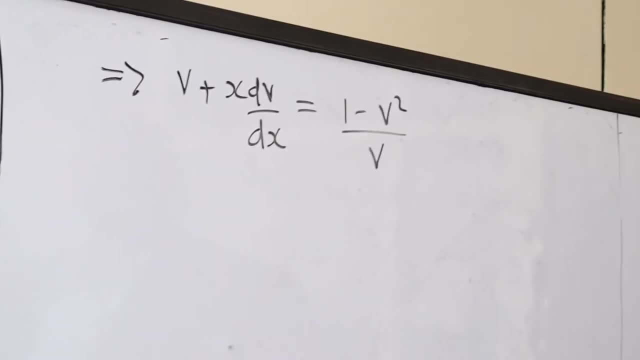 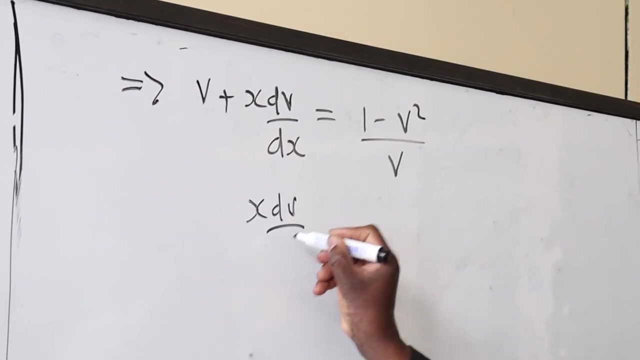 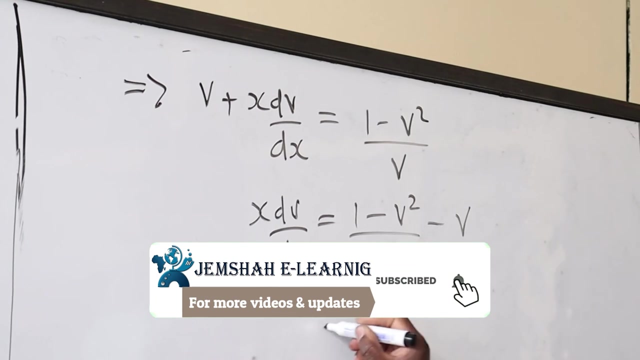 will be equal to 1 minus v, squared all over v. It will simplify to that Now. we want now to separate the variables, So we can say here: x, dv, dx will be equal to 1 minus v, squared all over v minus v. 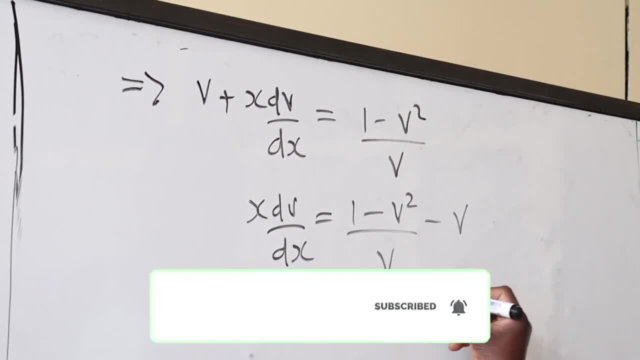 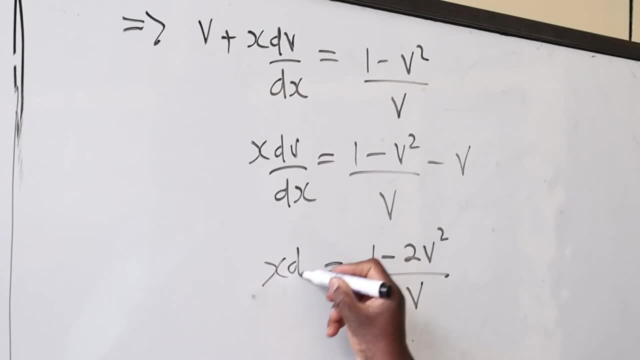 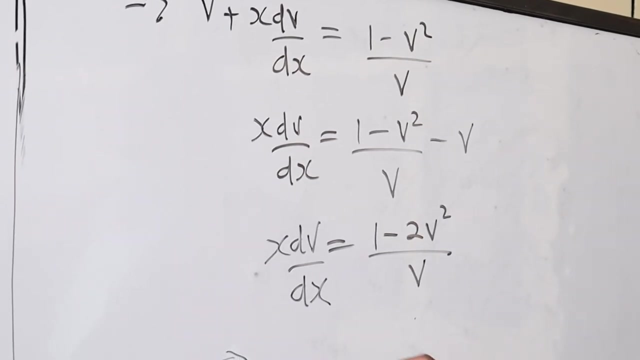 Which will be equal to 1 minus 2v, squared all over v x dv dx will be equal to that Which will be. this implies to now: dv v all over 1 minus 2v squared dv is equal to dx all over x. 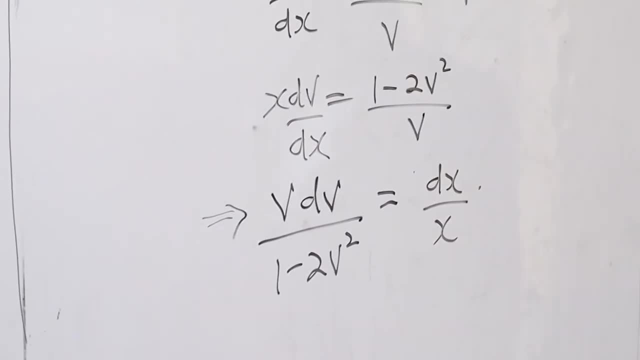 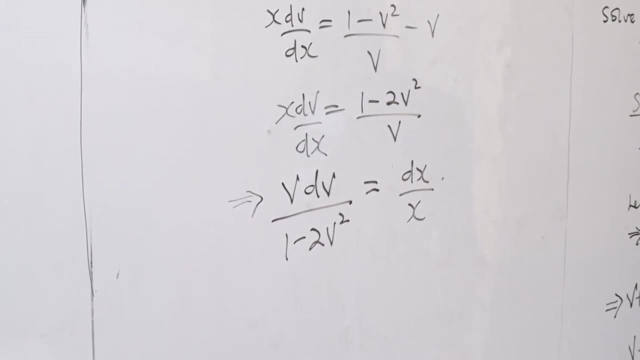 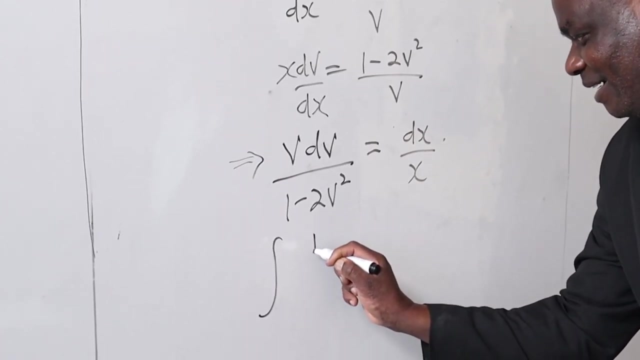 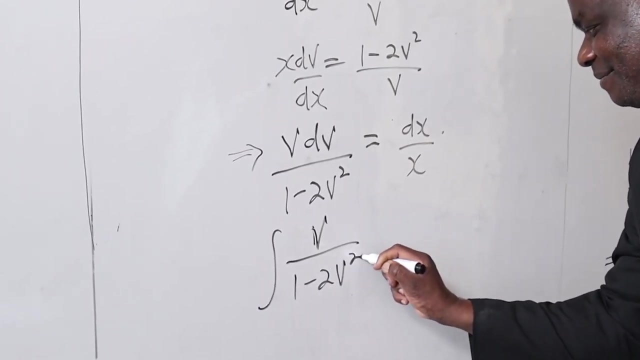 We have now separated the variables. Now, after separating the variables, to solve this ADD, we need only- we need only to integrate both sides with respect to the variable concerned. So this is 1 all over. this is the integral of v: all over, 1 minus 2v squared. 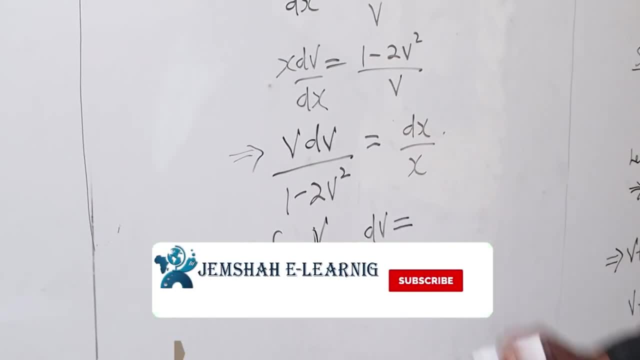 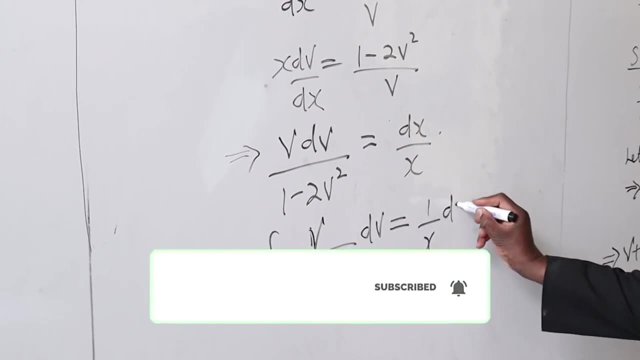 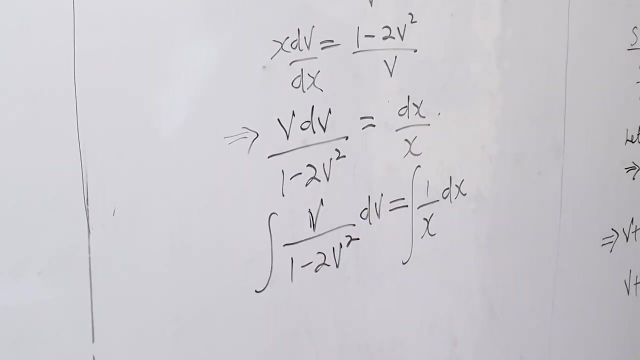 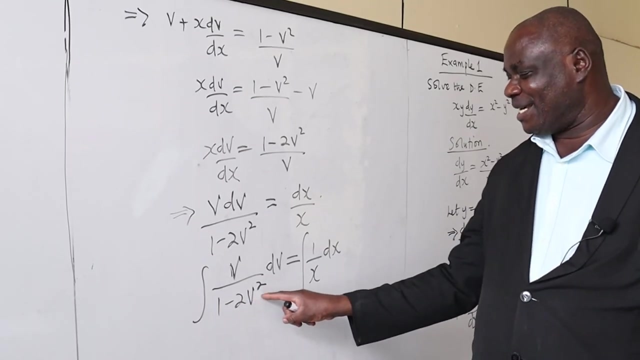 dv is equal to, is equal to dx all over x, Which is 1 all over x dx. So the integral of that. Now this is a quotient. We can now try to see whether, if we differentiate what we have in our denominator does, it gives us something that contains: 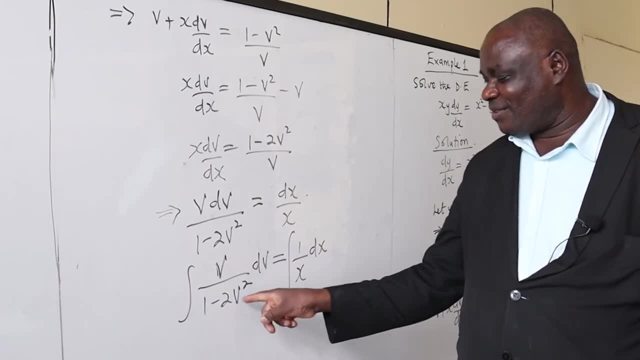 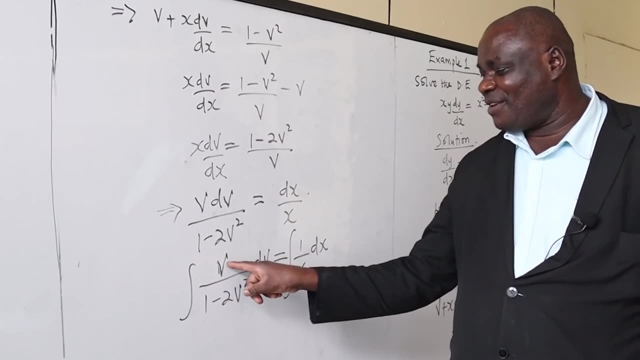 something in the numerator. So 1 minus 2v squared when differentiated with respect to v, we get negative 4v, And here we have v only. What is missing is a negative 4.. A constant can always be included if we like. 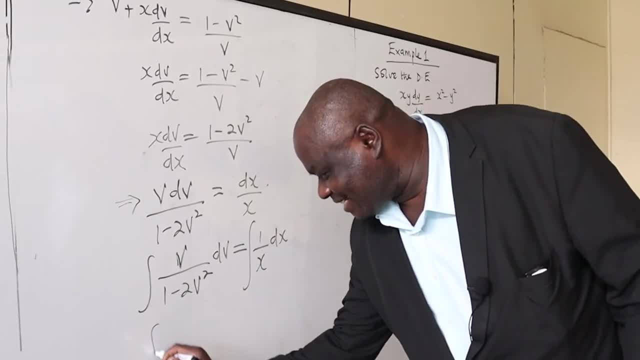 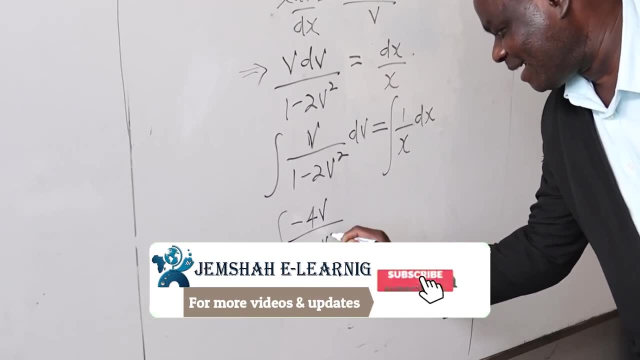 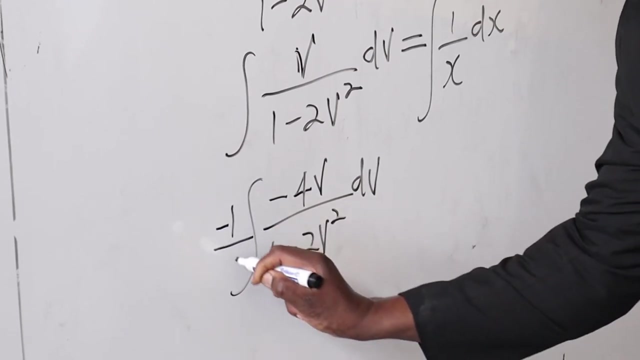 If it is going to help us. So we say this is the integral of minus 4v there, All over 1 minus 2v squared dv. and this one we say we remove that one, so it will be minus 1 all over 4.. 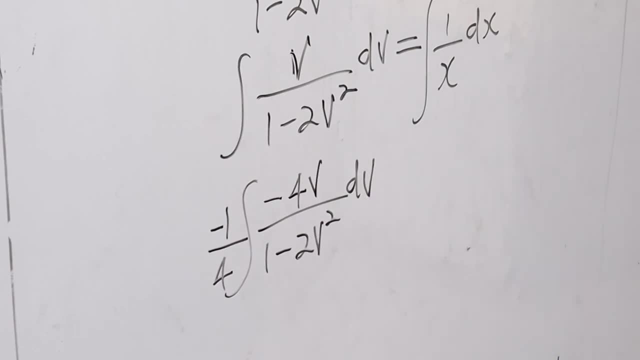 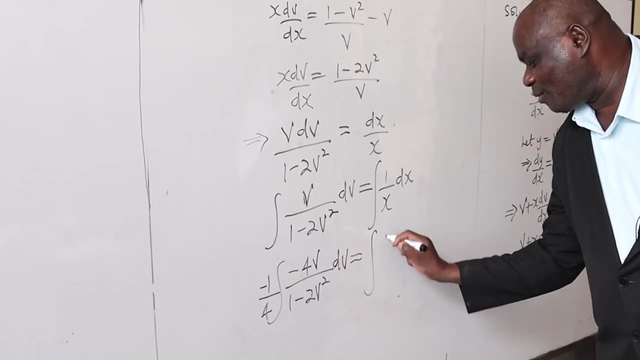 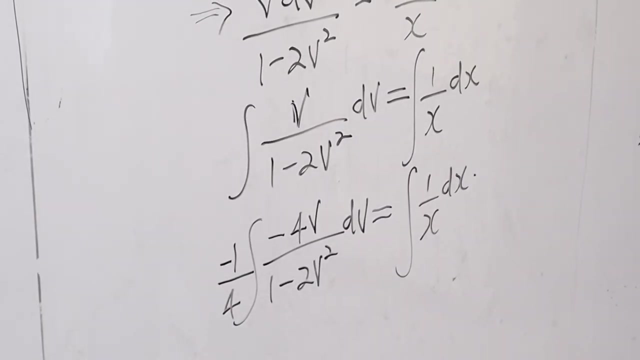 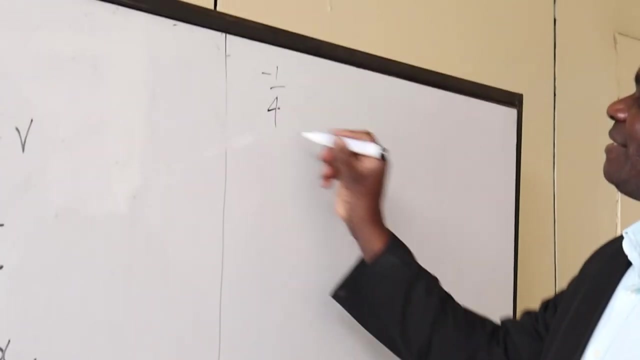 Minus 1 over 4. if you multiply by negative 4, you get 1, which was there before, which is 1.. It's equal to the integral of 1 all over x, dx. The same simplifies to minus a quarter ln of 1 minus 2v squared. 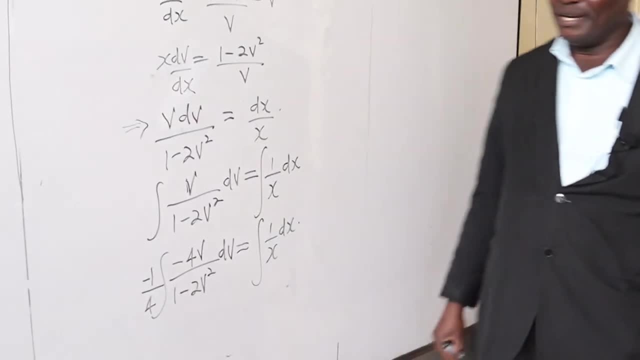 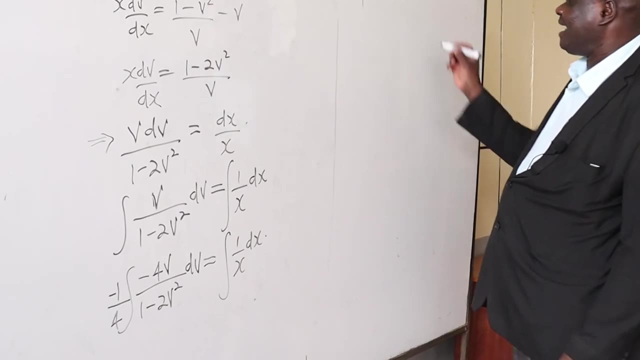 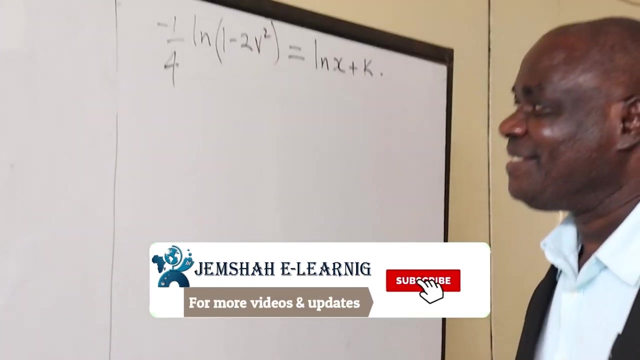 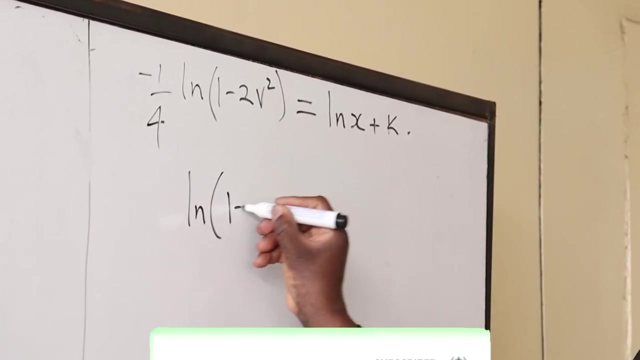 because the numerator is the derivative of the denominator. so the answer, when integrated, becomes ln of the denominator, Natural log of the denominator, which will be equal to ln over x plus a constant k. So this simplifies. now to ln of 1 minus 2v squared. 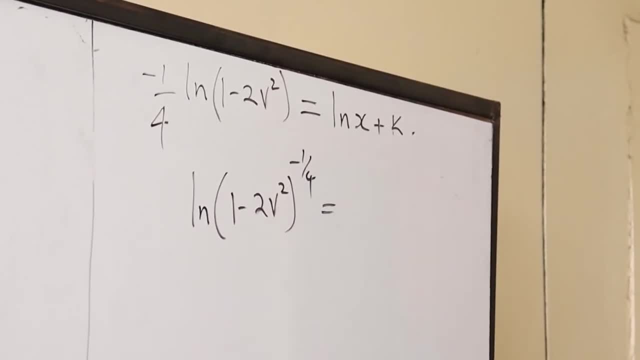 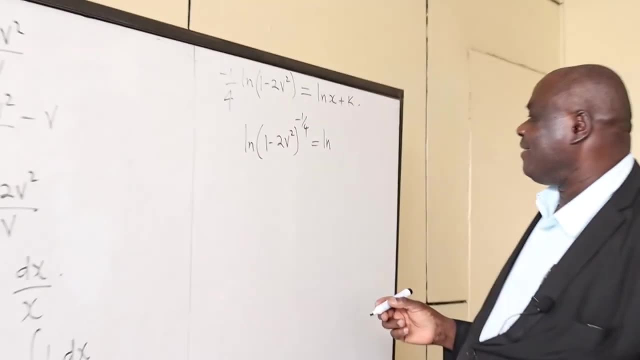 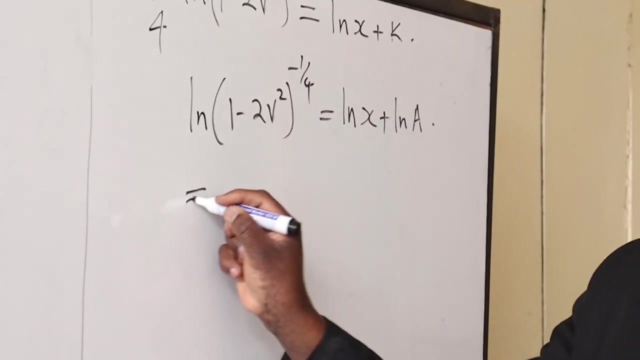 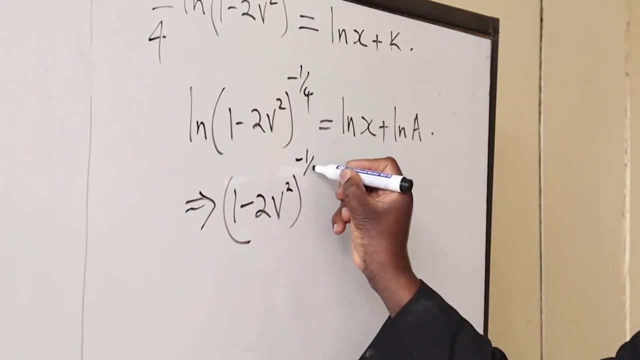 raised to power minus a quarter will be equal to ln. k can be ln of a, k can be ln of a. so this is ln of x plus ln of what a. This implies what 1 minus 2v squared, raised to power minus a quarter. 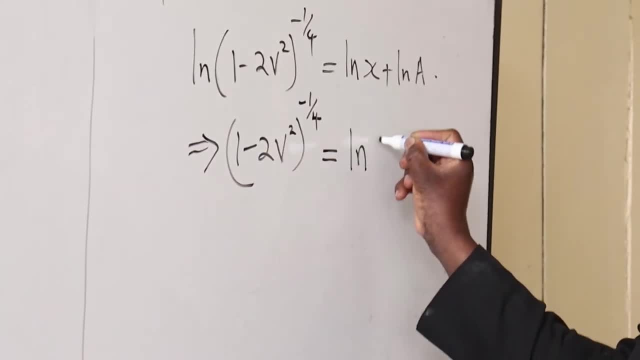 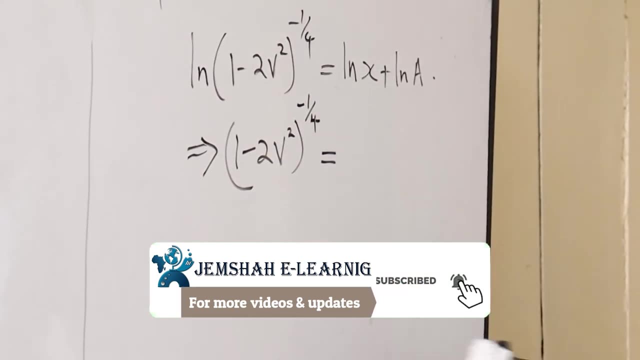 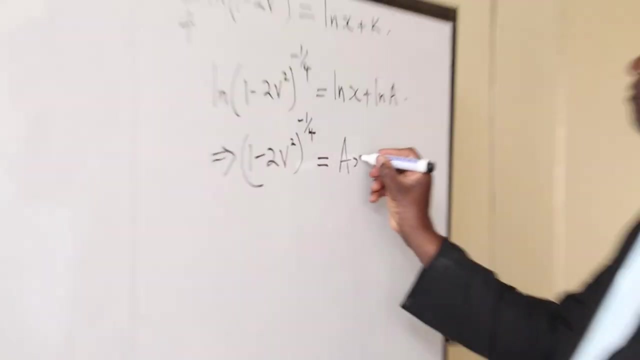 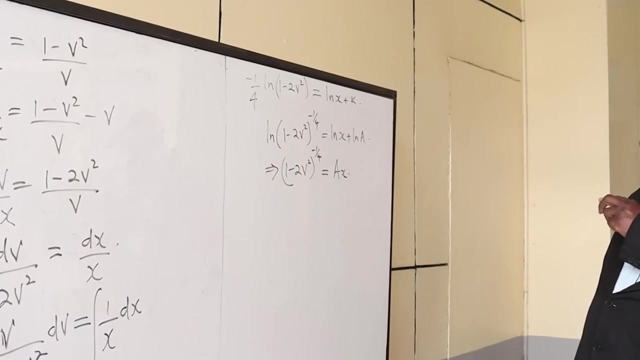 will be equal to ln of ax will be equal to. will be equal to ax will be equal to ax. Now, before. that is the solution to our differential equation after separating the variables, but it has v in it. we would like to substitute the value of v. 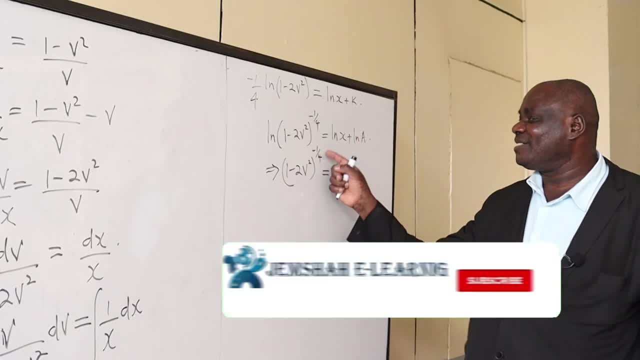 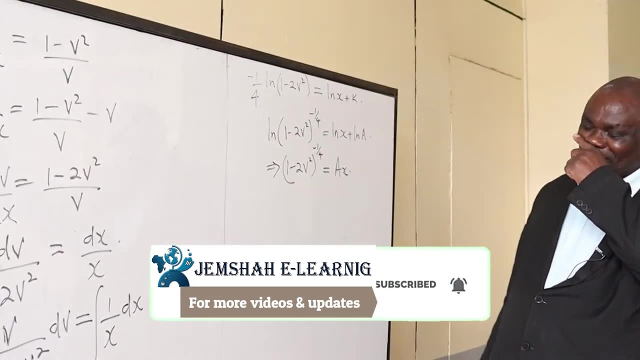 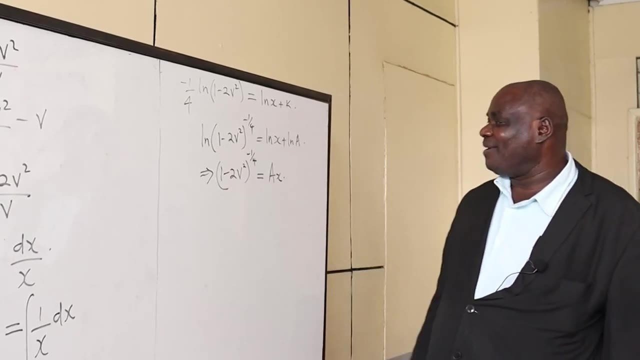 and before we do so we can clear this particular bit. This power negative a quarter, So power negative a quarter. that means we can raise both sides to a power 4.. Power negative 4. Or this one we can write as 1 all over. 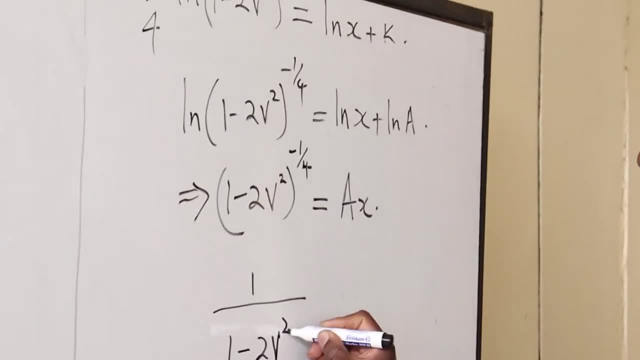 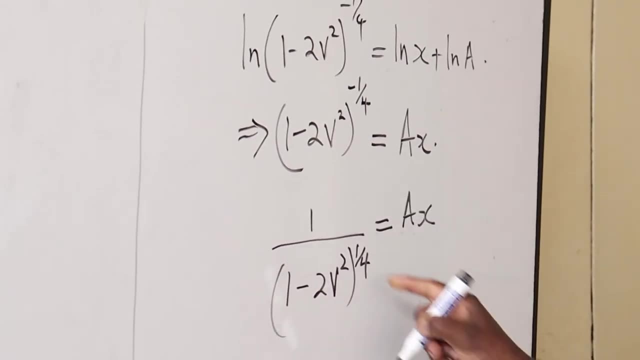 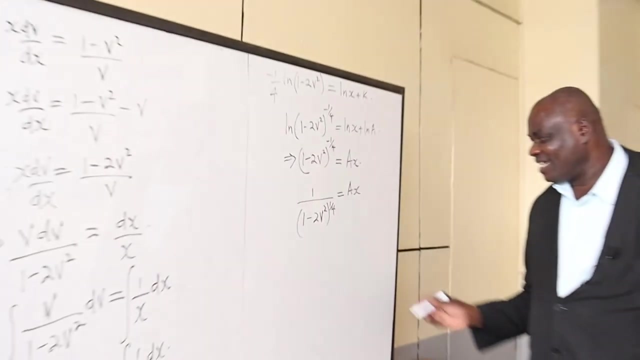 1 all over, 1 minus 2v squared. raised to power a quarter here is equal to ax. Now to clear power quarter. to clear power quarter, we raise both sides to power 4.. So this one will be 1 all over 1 minus 2v squared. 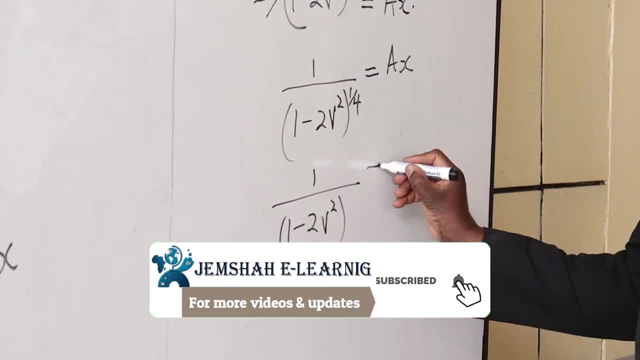 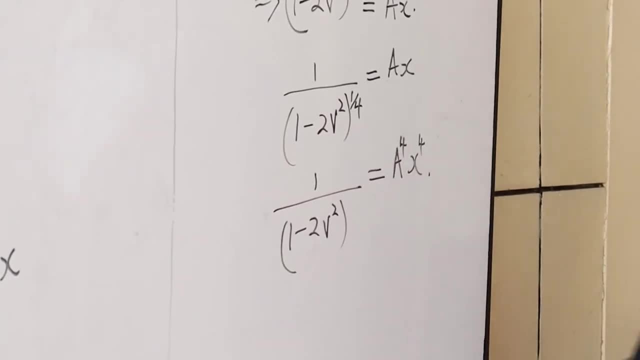 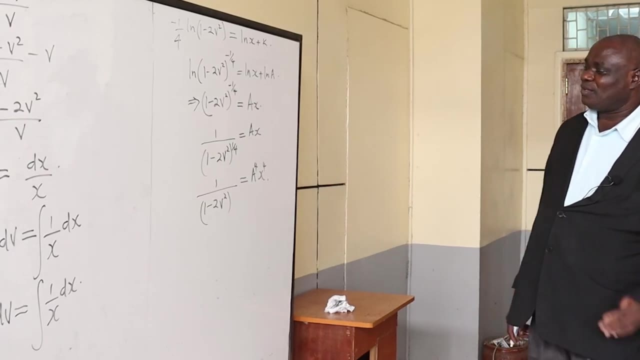 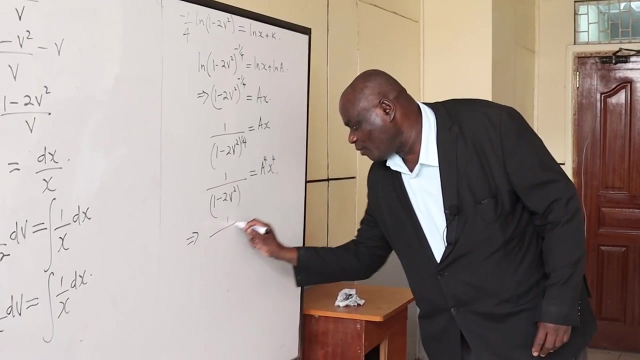 then power. now 1 will be equal to a power 4 x power 4. a power 4 x power 4. From here, then, we can now substitute for the value of v, So this implies 1 all over 1 minus 2 into y squared. 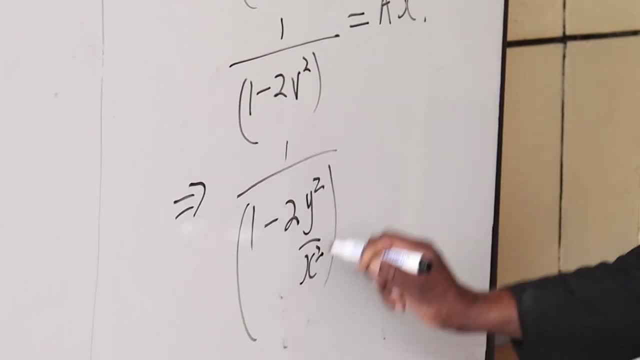 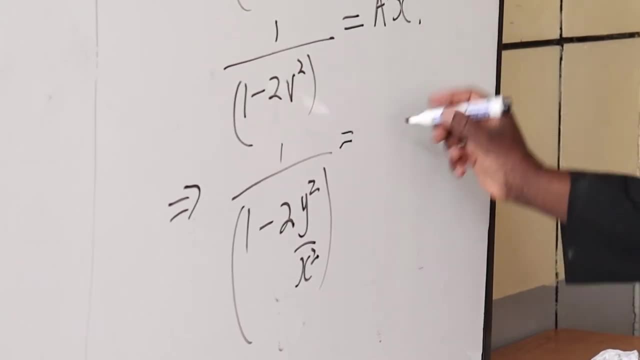 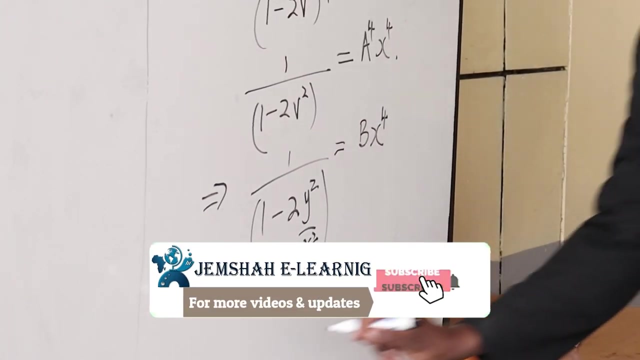 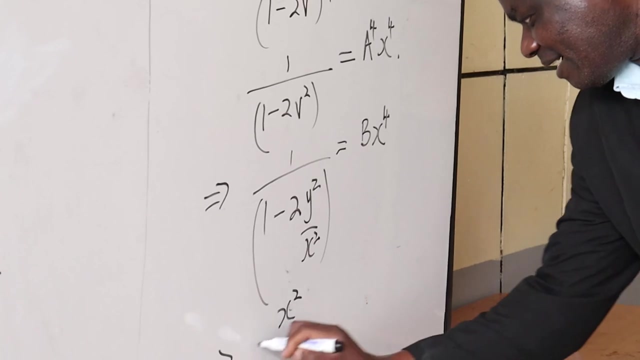 all over x squared, y all over x. when you square, you get y squared all over x squared is equal to a power. 4 can now be written as a new constant: b x power 4. So this implies what This gives us: x squared all over. 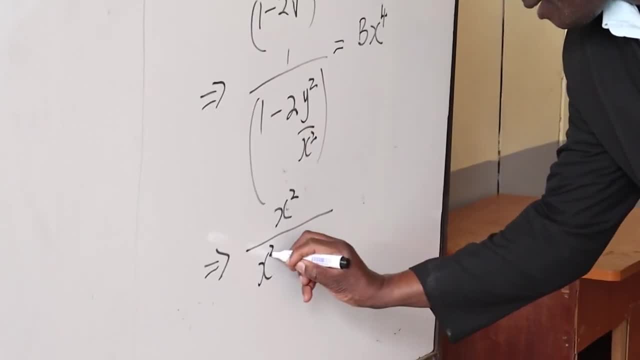 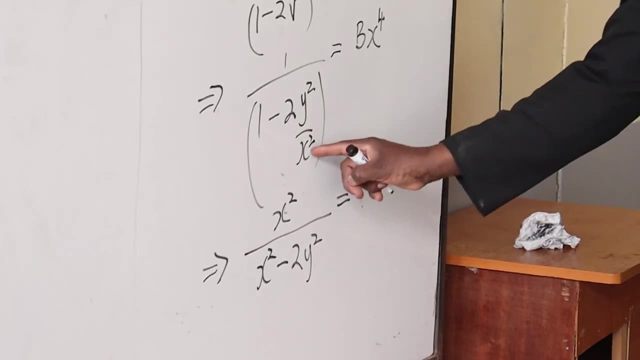 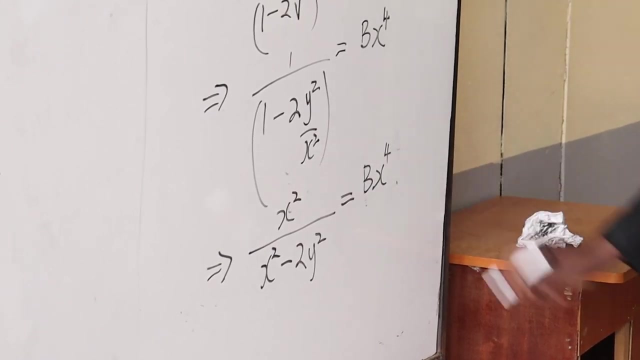 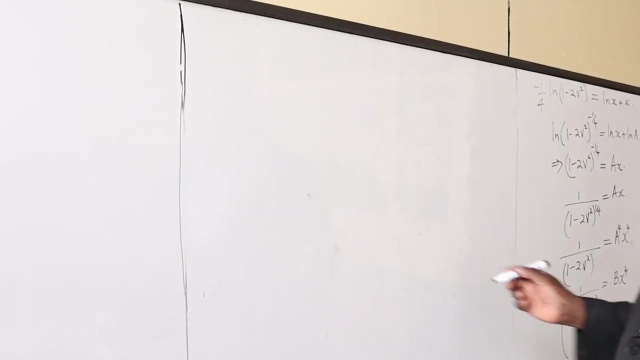 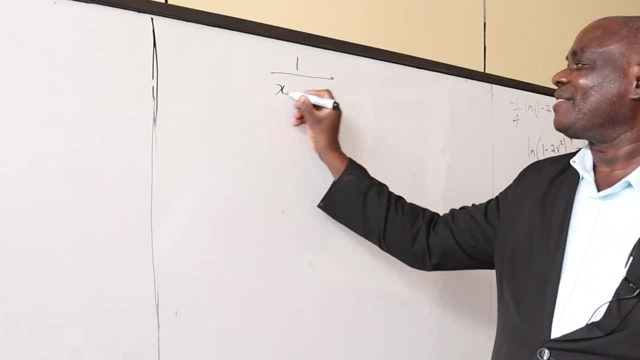 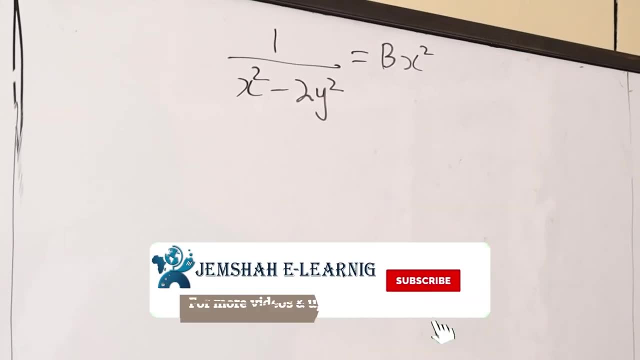 by x squared, then we remain with 1 all over, 1 all over x squared minus 2y squared minus 2y squared is equal to, is equal to b x squared, b x squared, b x squared. This implies, this implies what Cross multiplying what.